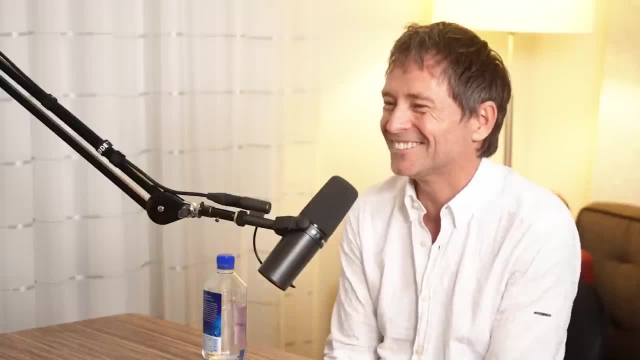 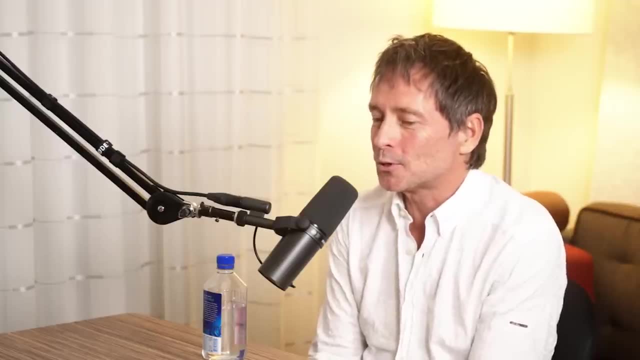 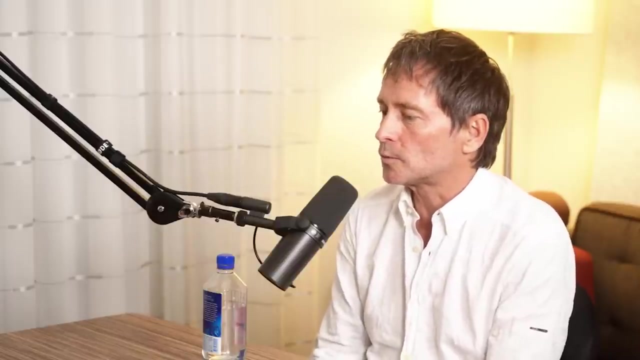 Well, yes, How much time do you have? We talked about time previously. Time is an illusion, right? So we agreed. So Kurt Gödel was a great Austrian mathematician and logician. He moved to the United States before the Second World War and worked at the Institute for Advanced Study in Princeton. 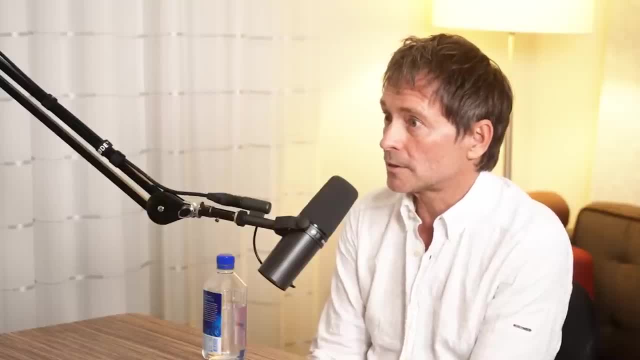 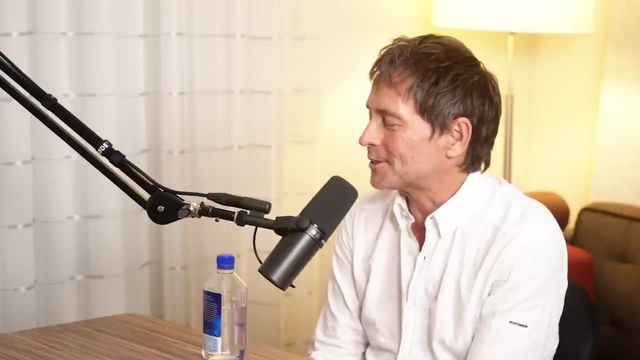 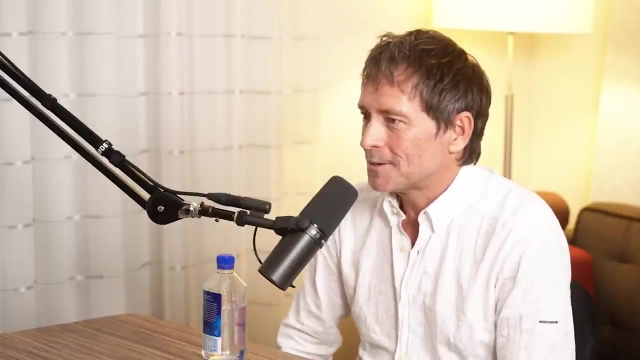 where he was a colleague of Einstein and other great scientists- von Neumann, Hermann Weil and so on. But one interesting quote that I like in this regard is that Einstein said that at some point he said that the only reason he came to the Institute was that he would have the privilege of walking. 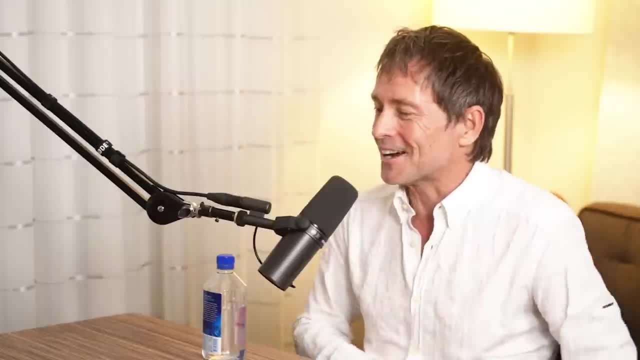 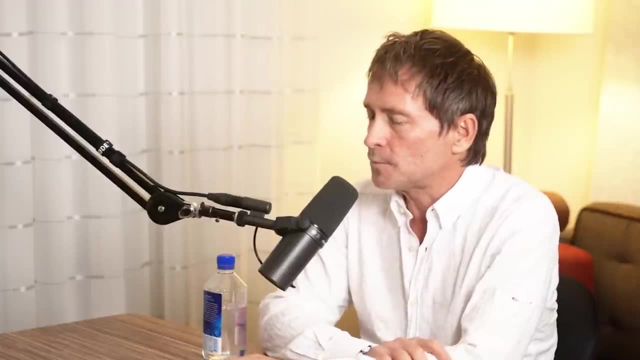 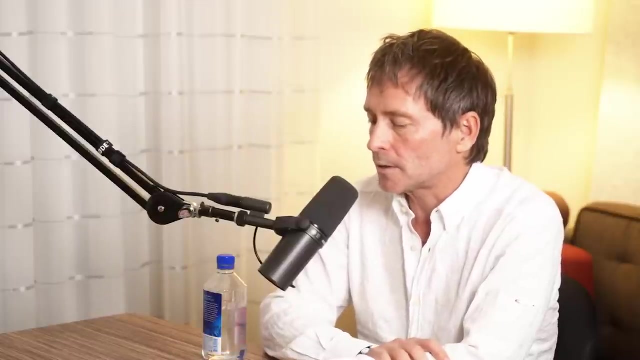 back home with Gödel in the evening. So in other words, Einstein thought that Gödel was the smart one. okay, So his most important contribution was his two incompleteness theorems: the first incompleteness theorem and the second incompleteness theorem. And what is this about? It's really a. 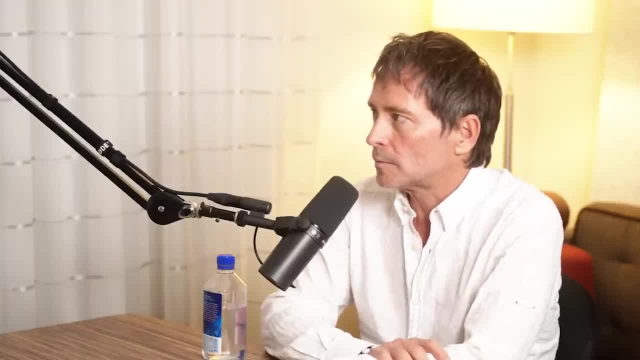 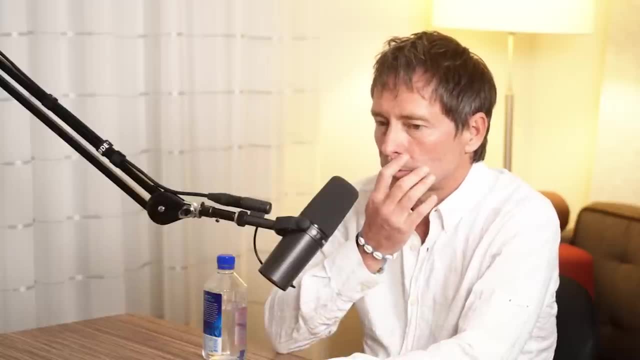 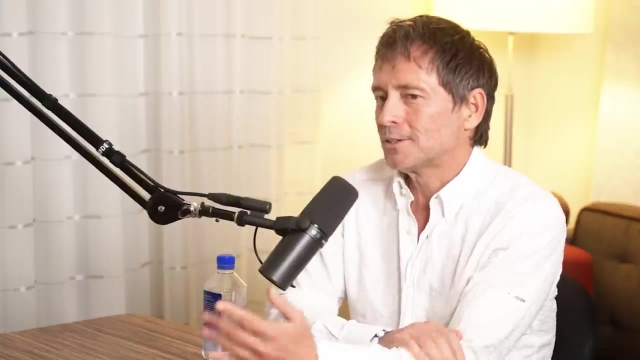 lot about inherent limitations of mathematical reasoning, the way of producing mathematical theorems, the way we do it. So, to set the stage, how do we actually do mathematics? So we know that we discussed that, say, physics is based on mathematics. and you could say: 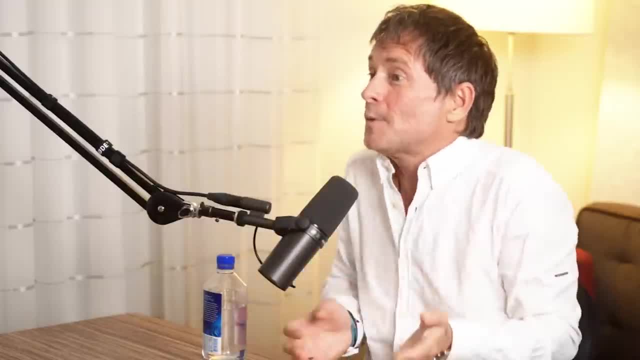 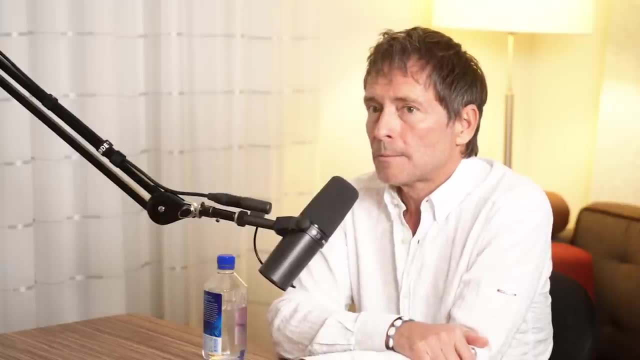 chemistry is based on physics, biology is based on chemistry. Okay, so it comes to mathematics. What is mathematics based on? Well, mathematics is based on the fact that we have to learn to divided by axioms, So any field of mathematics can be presented as what is called the formal system And, at the core, 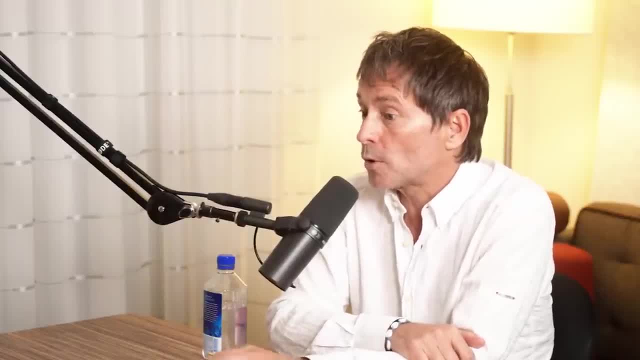 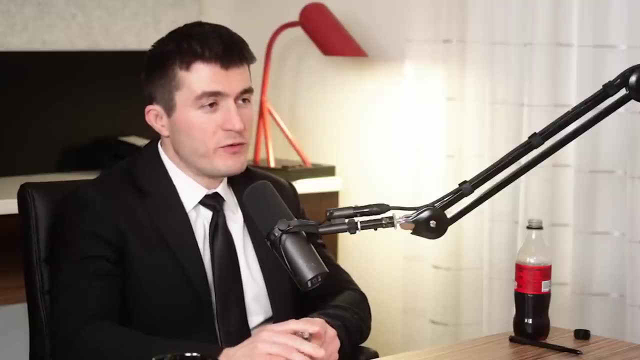 of the formal system is a system of axioms or postulates. These are the statements which are taken for granted, Given without proof. Without proof, An example would be so that one of the very first formal systems was the system was Euclidean geomancy. Exactly So to get the Euclidean geomaniac, if you take the imperialism. 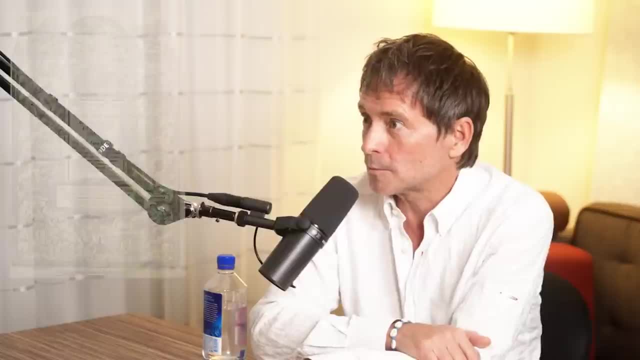 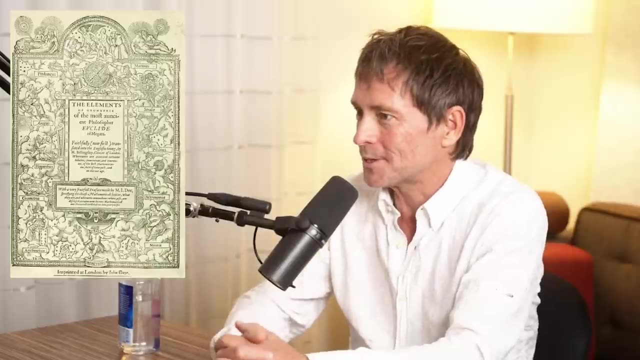 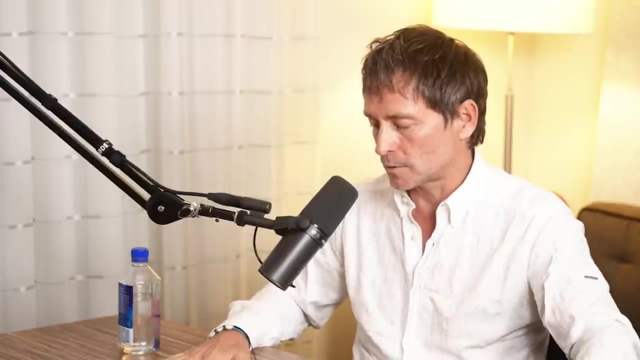 developed by Euclid in his famous book Elements about 2,200 years ago. It's a subject familiar from school because we studied it, but what it's really about is the geometry of the plane Plane. by plane I mean just this tabletop extended to infinity in all directions. 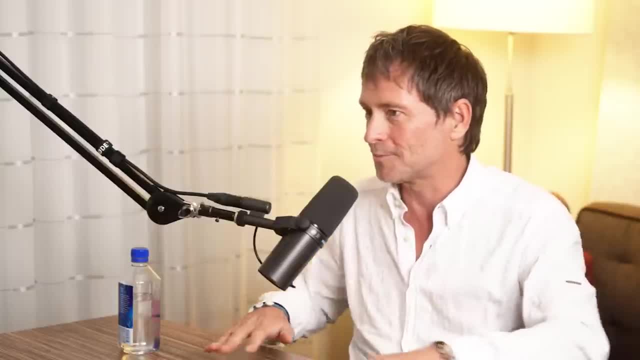 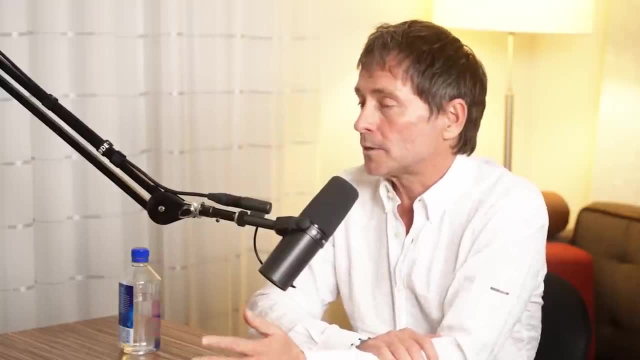 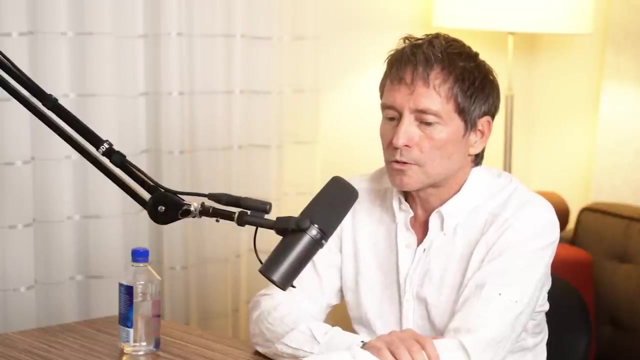 kind of a perfect plane, a perfectly even table. Euclidean geometry is about various geometric figures on the plane, specifically lines, triangles, circles, things like that. So what's an example of an axiom? An example of an axiom is that if you have two points, 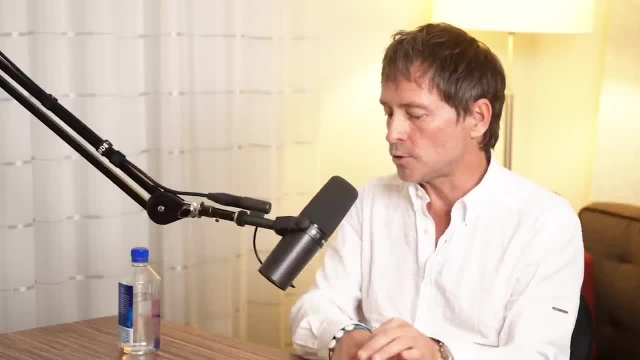 which are distinct, two points on the plane, then there is a unique line which passes through them. Now, kind of of an example of an axiom is that if you have two points which are distinct, two points on the plane, then there is a unique line which passes through them. Now, kind of. 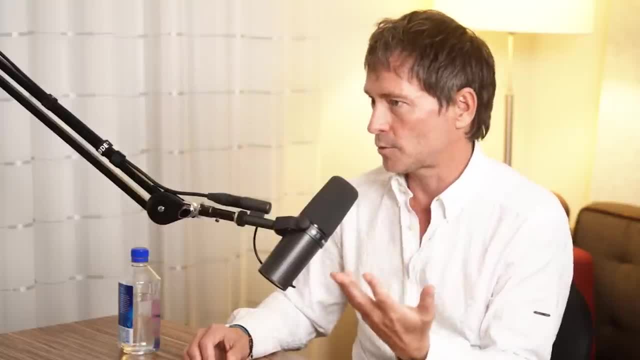 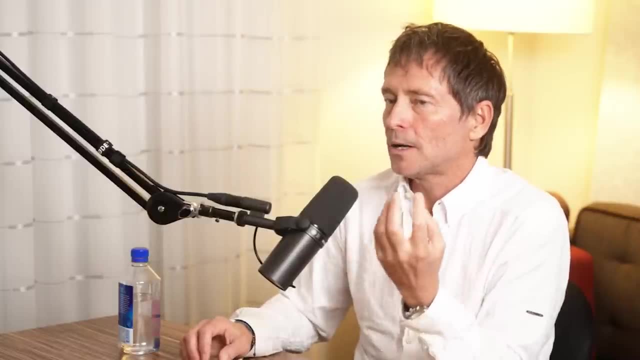 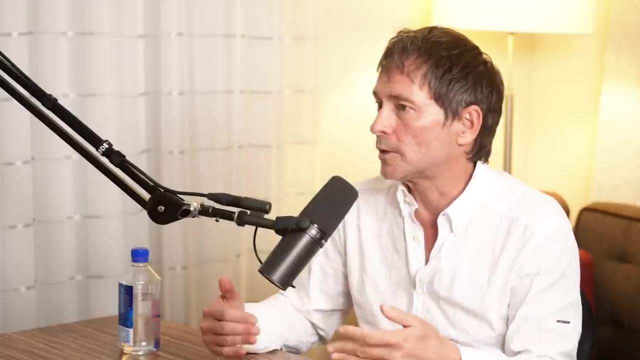 sounds reasonable, but this is an example of an axiom In mathematics: you have to have a seed, so to speak, You have to start with something, and you have to choose certain postulates or statements which you simply take for granted, which do not require proof. 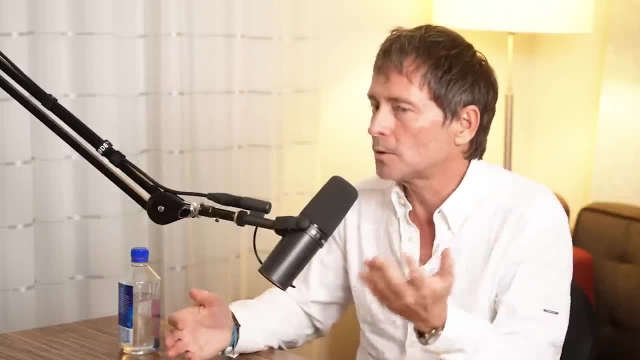 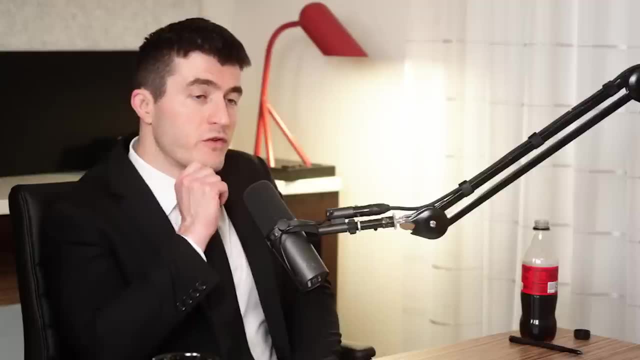 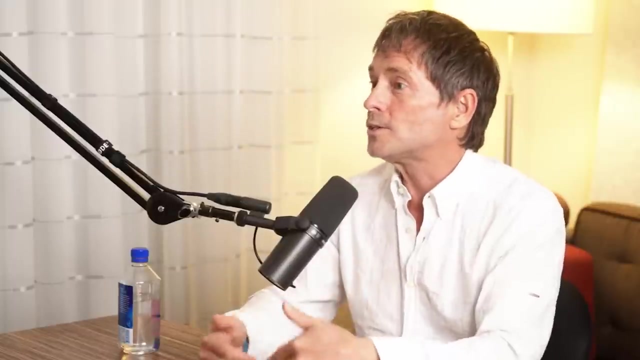 Usually they are ones which kind of intuitively clear to you. but in any case you cannot have any mathematics without choosing those axioms, And you refer to those as the observer because they're kind of subjective. The observer comes in the process of choosing the axioms. Who chooses the axioms? 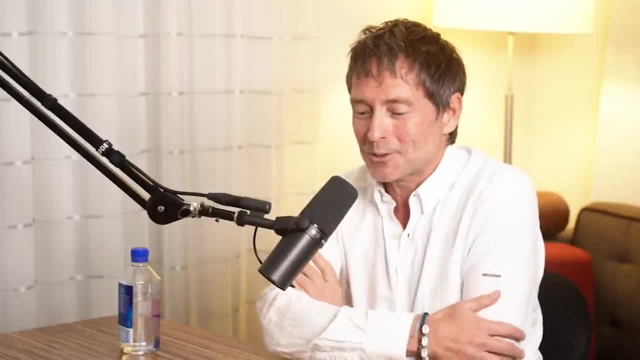 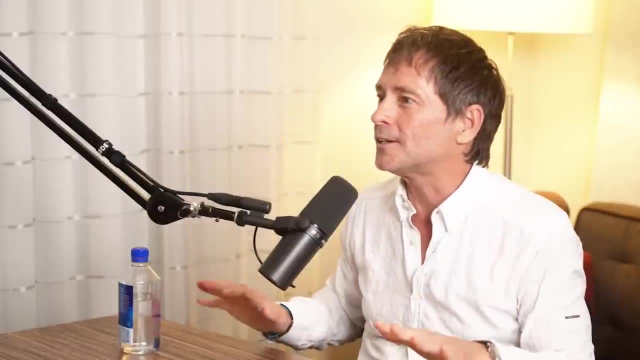 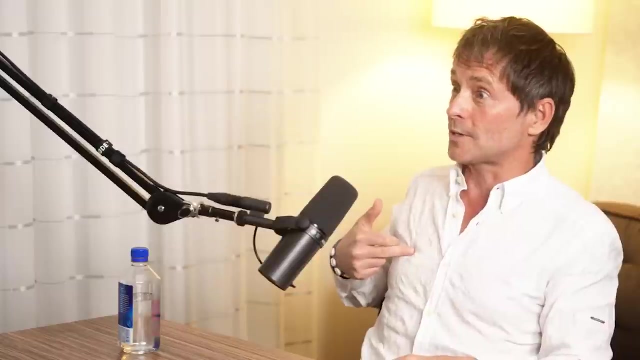 The turtles that it's all sitting on top of, As Alan Watts likes to say, who is watching the watchers? Yeah, And so in mathematics. but you see, mathematicians are so clever. It's really kind of like a little kind of a game of mirrors that we often like to say, and I used to say that that mathematics is a. 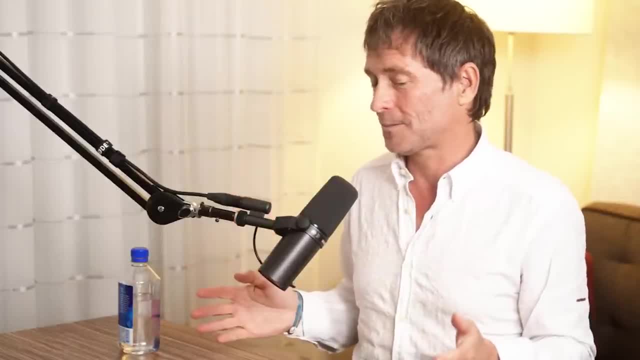 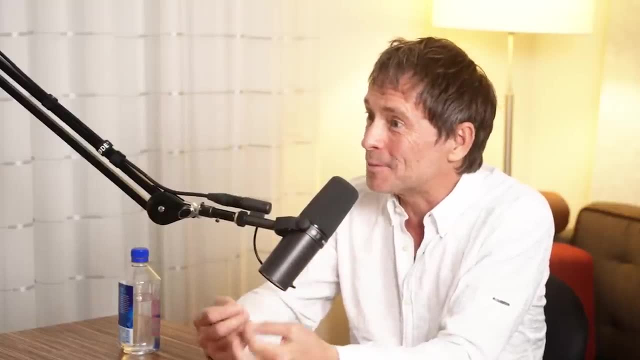 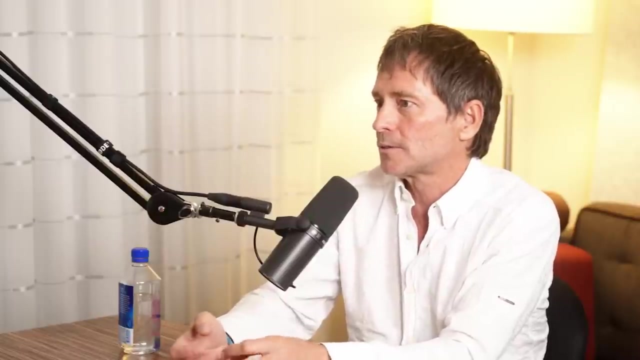 objective. It's really the only objective science, But that's because we hide this fact that actually is based on axioms, And the fact that there is no unique choice, that there are many choices, And so Euclidean geometry is actually a good illustration of this. 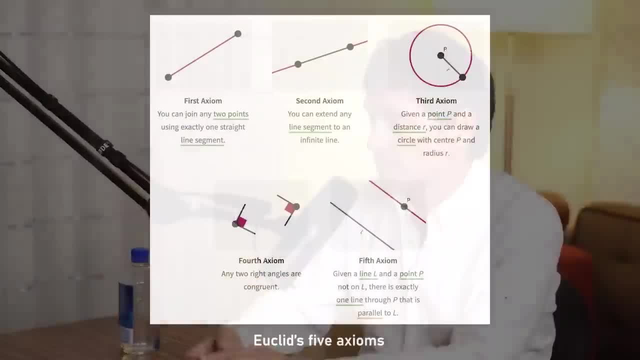 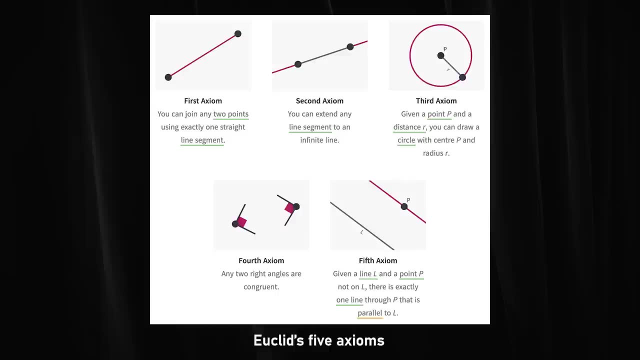 because Euclid had five axioms. Four of them were kind of obvious, like the one I just mentioned, And the fifth, which came to be known famously as the fifth postulate, was that if you have a line and you have a point outside of this line, 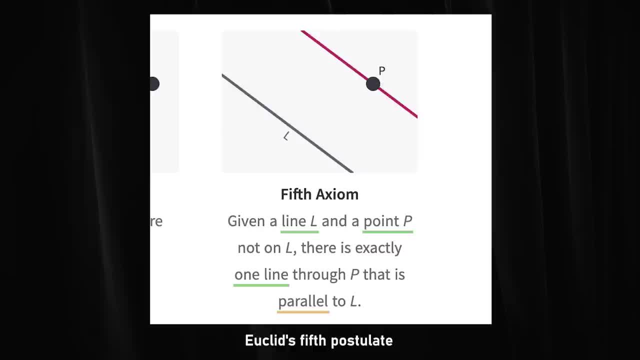 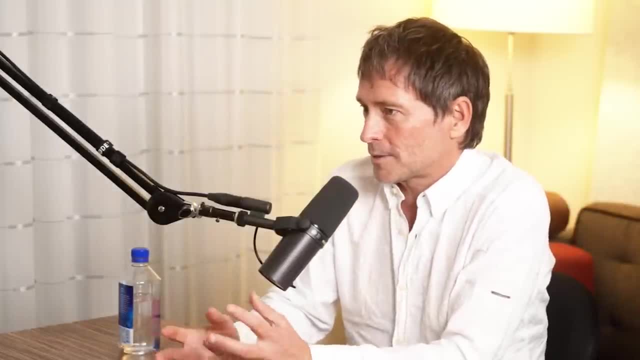 there is a unique line passing through that point which is parallel to the first line, meaning that it doesn't intersect, And Euclid himself was uncomfortable about this because he felt that it was kind of you know, he takes for granted something that is not obvious. 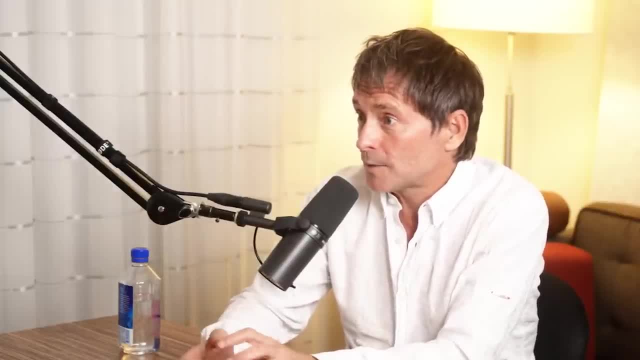 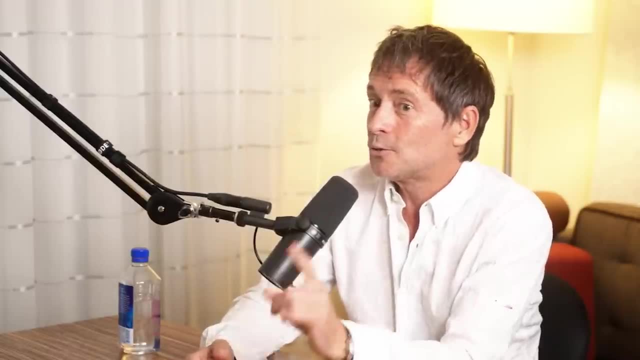 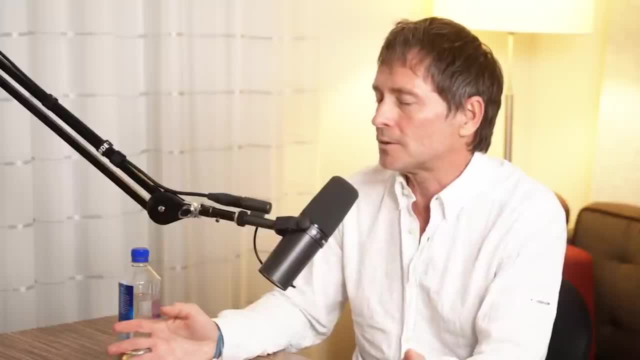 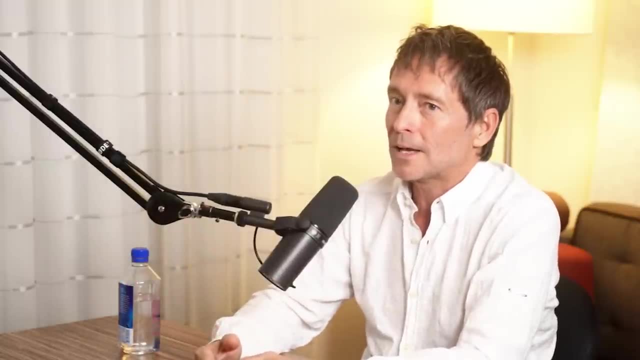 Which of course sounds very complicated, but it's not. Think of a sphere, just the surface of a basketball or the surface of the Earth. idealized The analogs. so you have points, you have analogs of lines which are meridians. Every two meridians intersect, unlike parallel lines on a flat space, There is also a so-called hyperbolic plane where there are infinitely many lines which do not intersect. Yeah, So every possibility can be realized. there are different flavors. 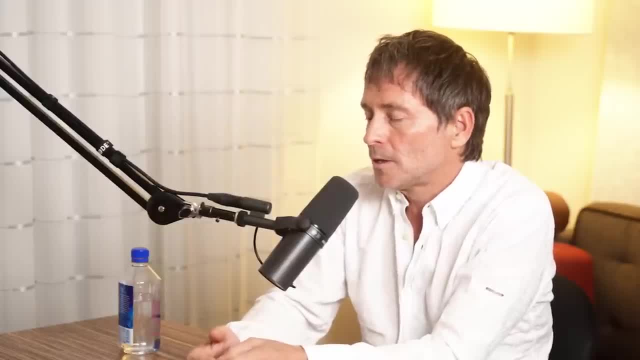 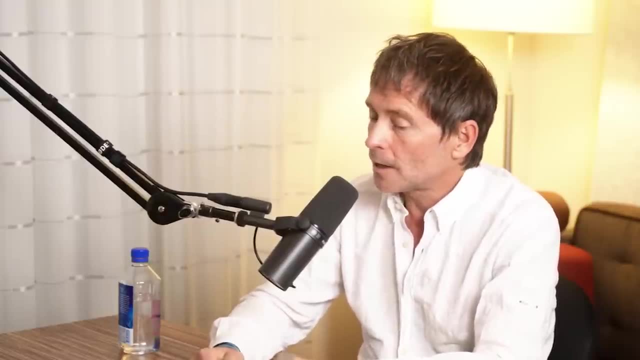 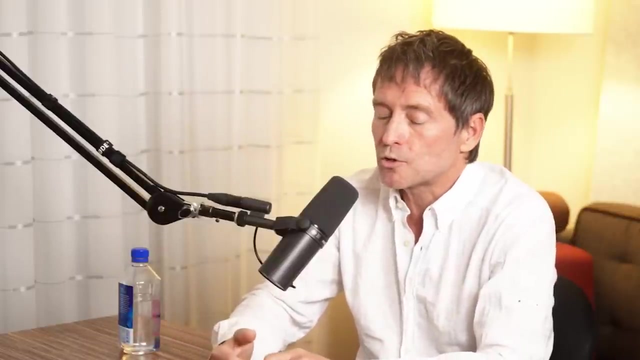 This is a good illustration of what a formal system is. You start with a set of axioms, those statements that you take for granted, and this is where you have a choice, and by making different choices you actually create different mathematics. After that, there are rules of inference, logical rules, such as if A is true and A. 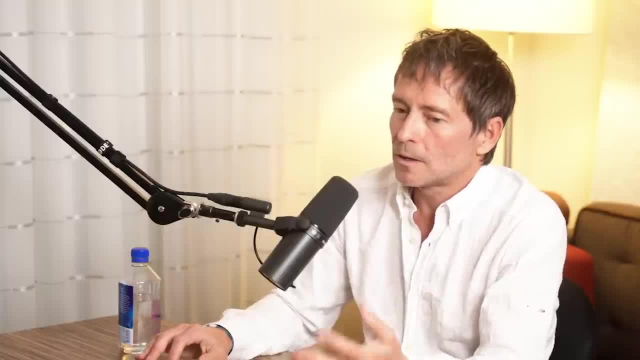 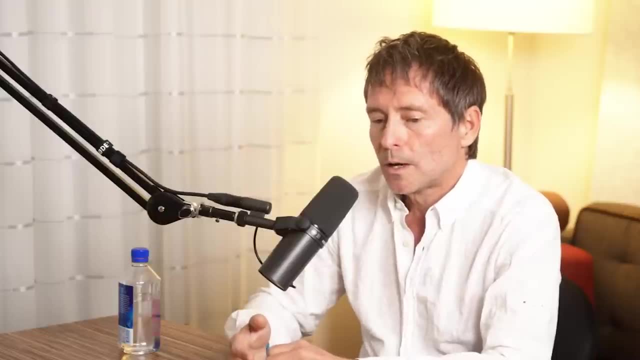 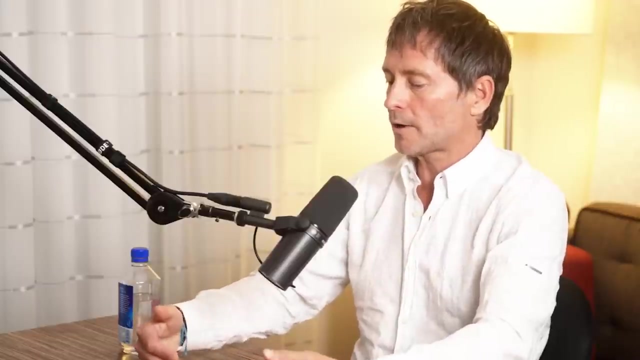 implies B, then B is true. Most of them were actually Introduced already by Aristotle, even before Euclid. And then it runs as follows: You have the axioms which are accepted as true statements, then you have a way to produce. 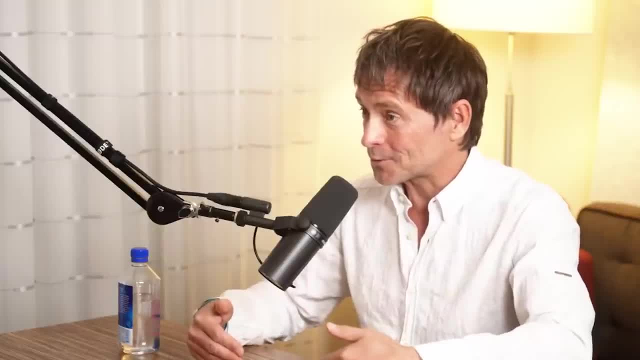 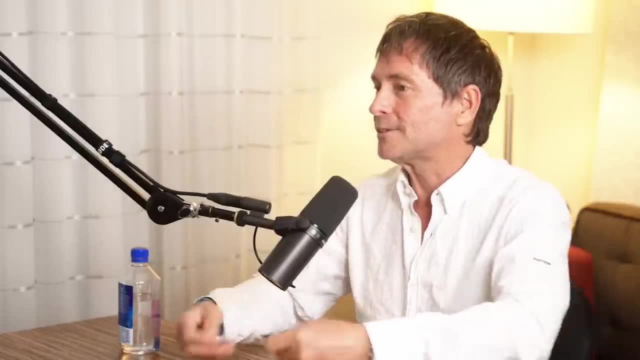 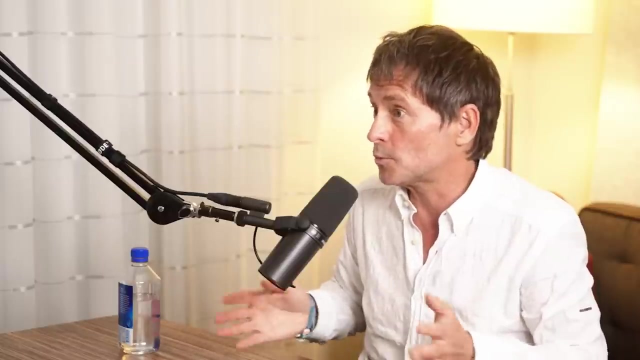 new statements by using the rules of logical inference from the axioms. Every statement you obtain you call a theorem and you kind of add it to the collection of true statements. And then the question is: how far can you go? How many statements can you prove this way? 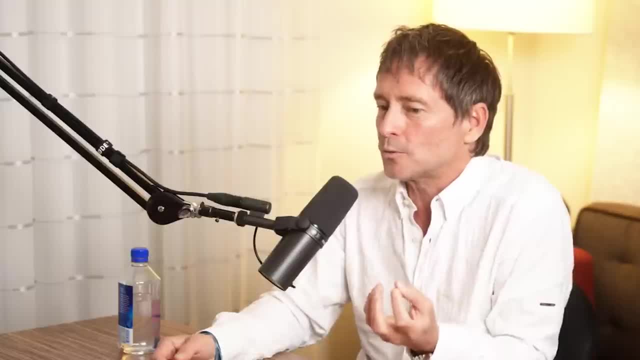 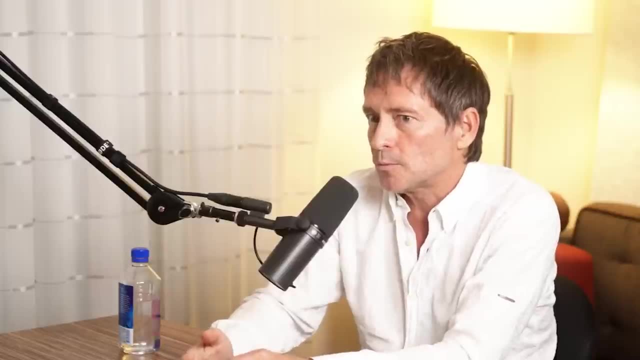 Of course you want the system to be non-trivial in the sense that you don't prove everything, Because if you prove everything, it would mean that it's self-contradictory that you prove a statement A and it's negation. 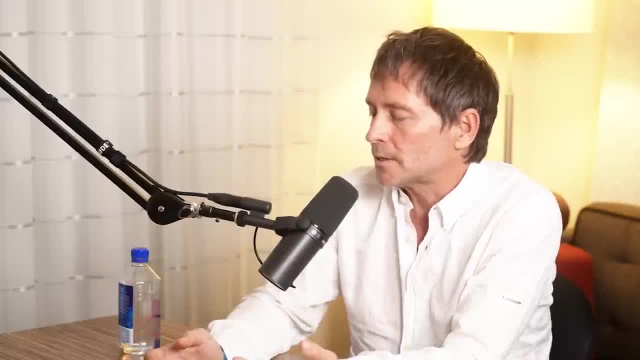 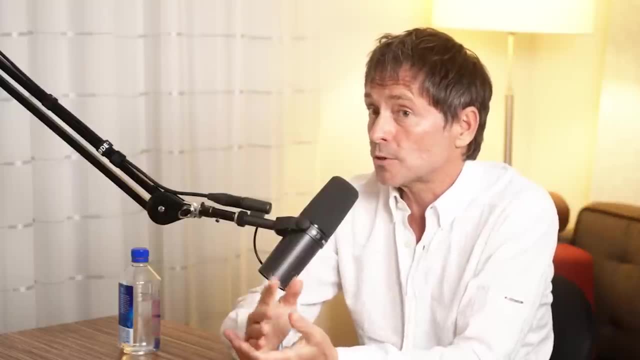 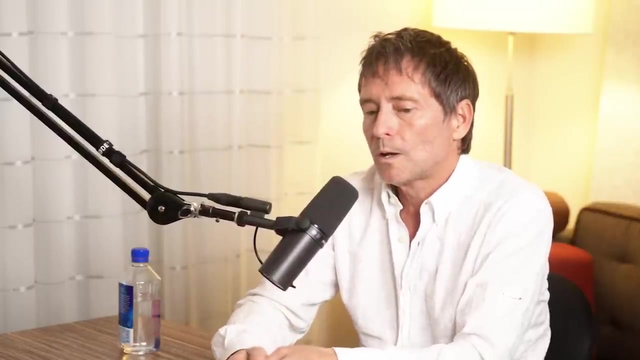 So that's kind of useless. It has to be discriminating enough so that it doesn't prove contradictory statements. So there is already a question of that mathematicians call consistency. it has to be consistent in the sense that it is not self-contradictory. 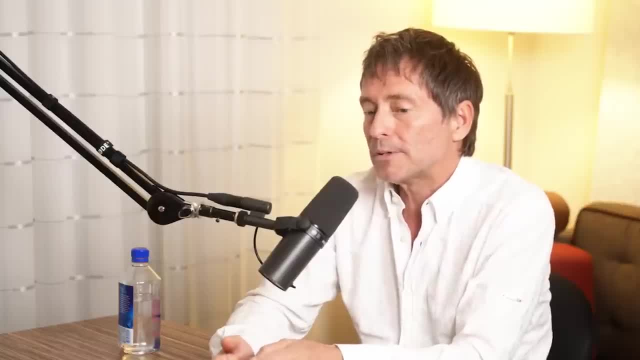 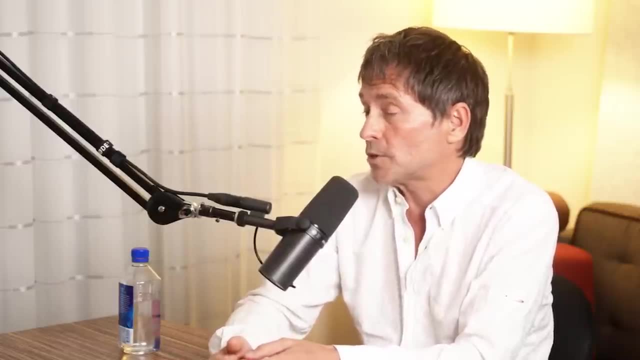 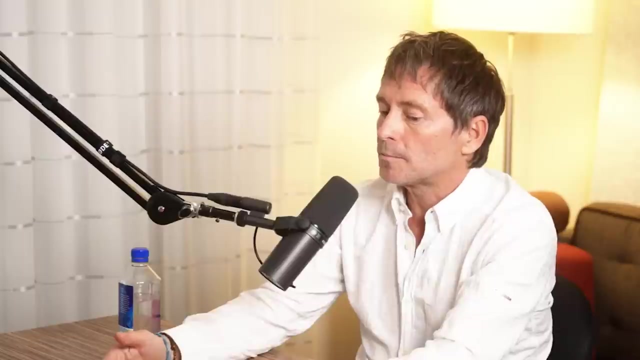 And then the idea that was basically prevalent in the world of mathematics by the beginning of the 20th century was that, in principle, all of mathematics could be derived this way. We just have to find the correct system of axioms, and then everything you ever need. 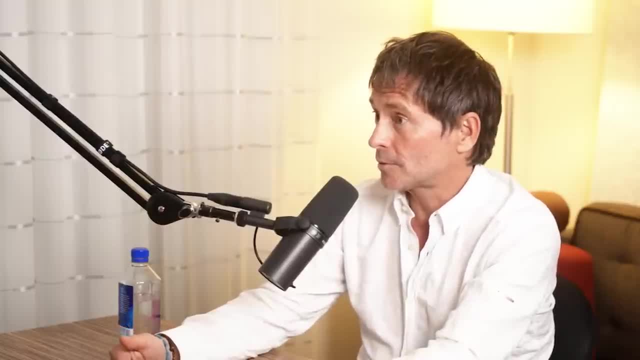 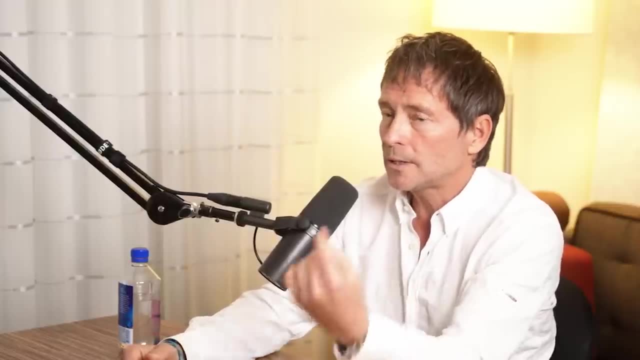 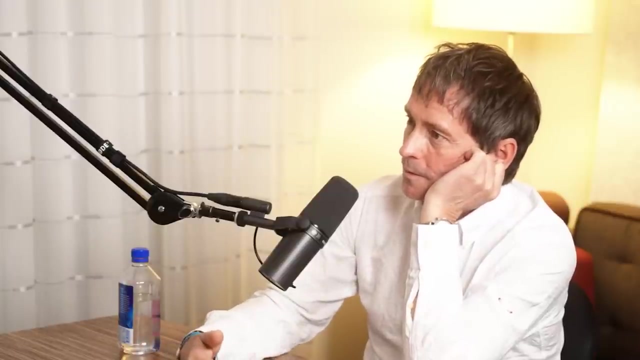 could be produced by this procedure, which is really algorithmic procedure, which actually could be run on a computer. Now think about it. What is special about this process? In this process, you are just manipulating symbols. basically, You're going from one statement to another without really understanding the meaning of. 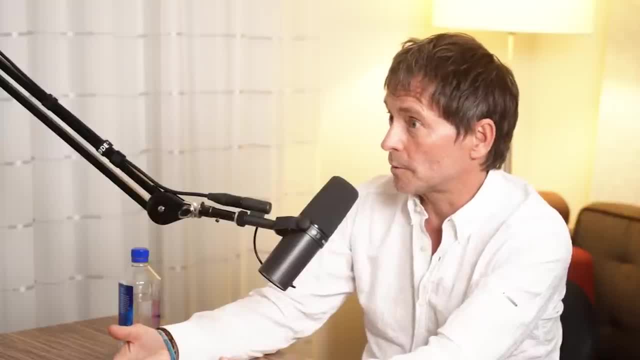 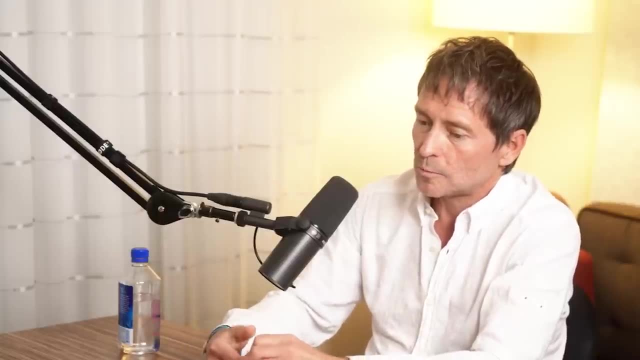 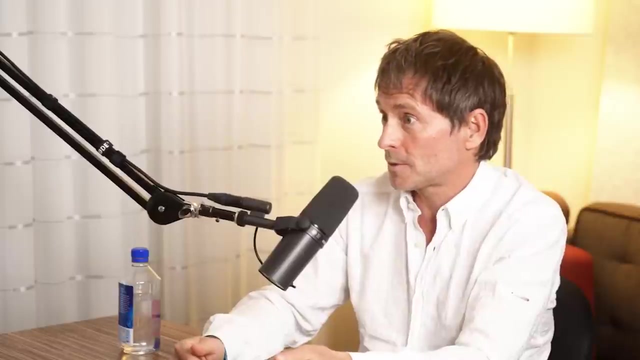 it, So it's an ideal playground for a computer program. It's a purely syntactic process where there are some rigid rules of passing from one statement to the next. Most mathematicians believed that this way you can produce all true statements. 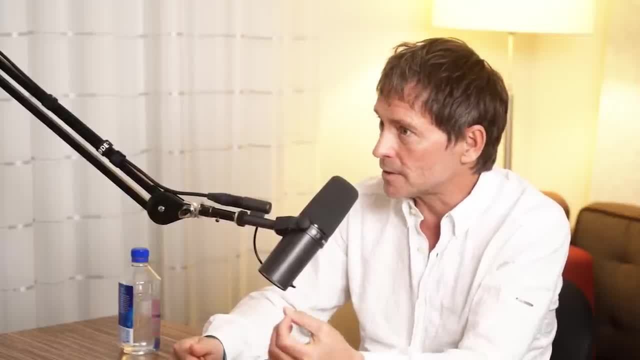 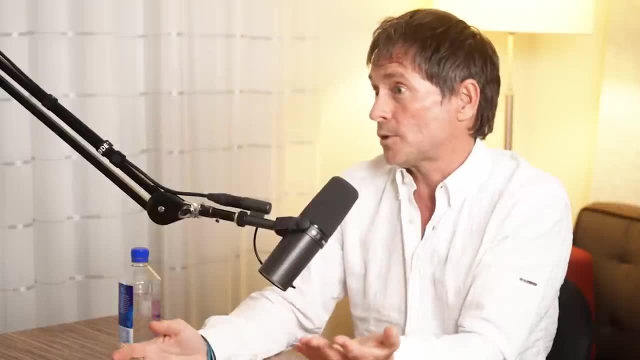 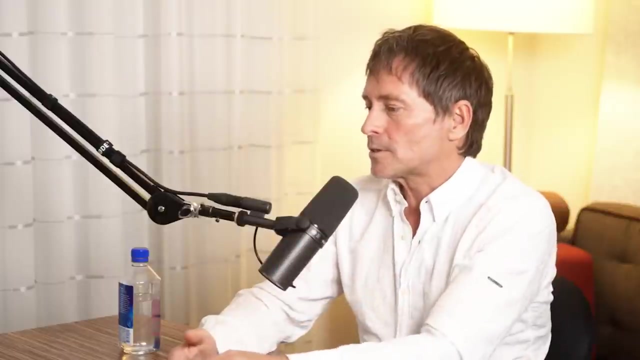 And if this were true, it would give a lot of credibility to the thesis that everything in life is computational or life is computation, Because then at least mathematics is computational, because then it can be programmed, and a computer, after sufficient time, depending on its capacity, would produce every true statement. 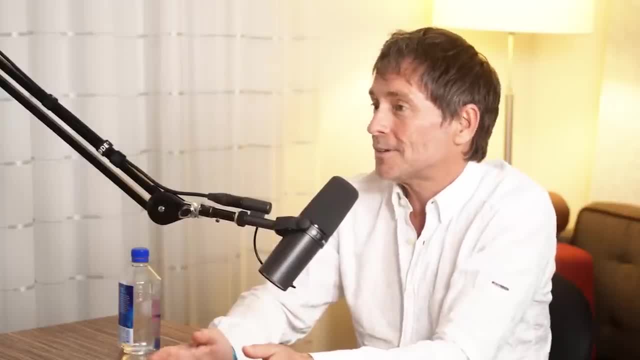 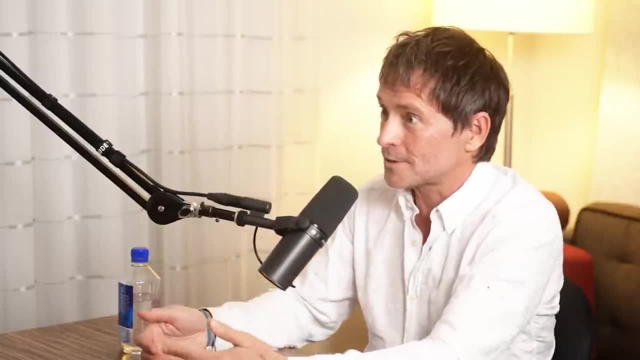 So Gödel's first incompleteness theorem says that that's not the case. And it not just says it, but it proves it at the highest level of rigor that is available in mathematics, That is to say within another formal system that he was operating in. 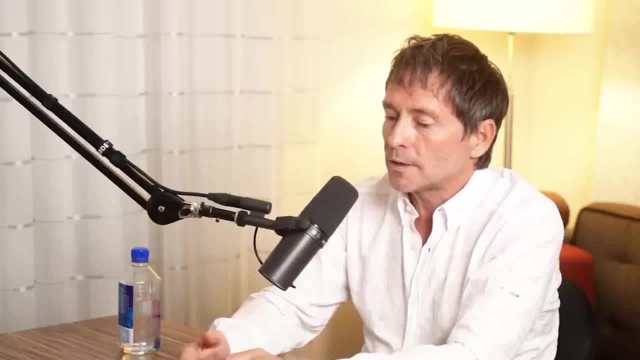 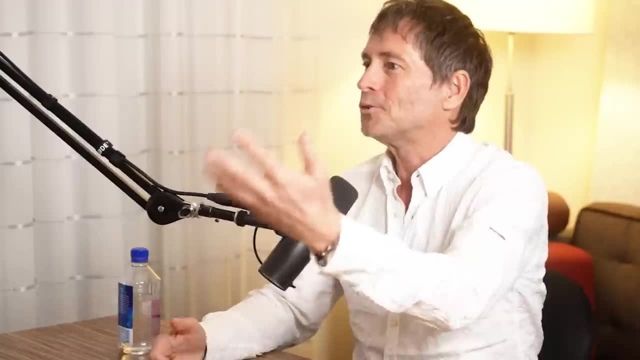 So, more precisely, what he proved was that if you have a sufficiently sophisticated formal system, that is to say that you can talk about numbers, whole numbers in it, that you have whole numbers one, two, three, four, you have formalized the operation of addition. 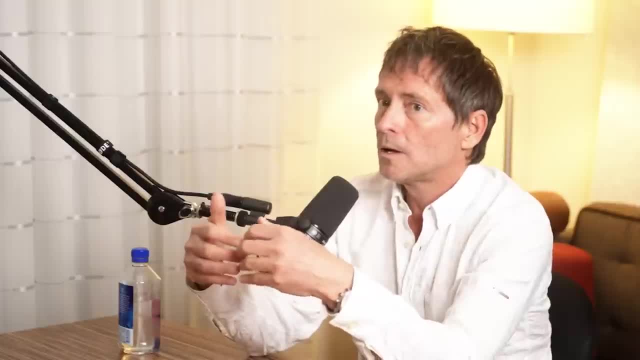 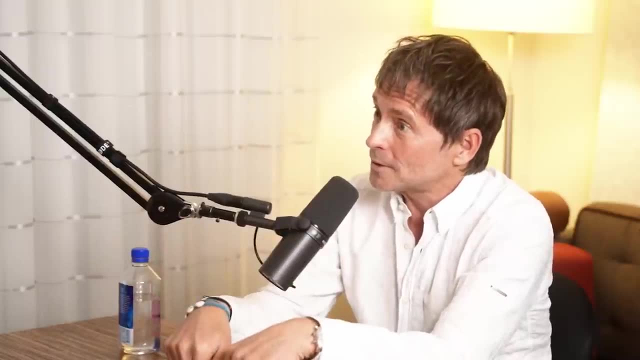 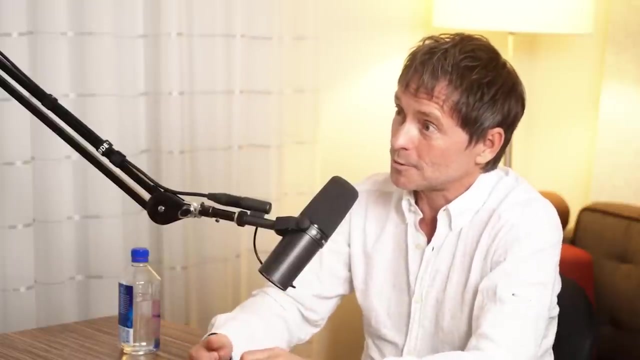 and multiplication Within the system. If it is consistent, that is to say if it's not completely useless, then there will be a true statement in it, which cannot be derived by this linear syntactic process of proving theorems from axioms. 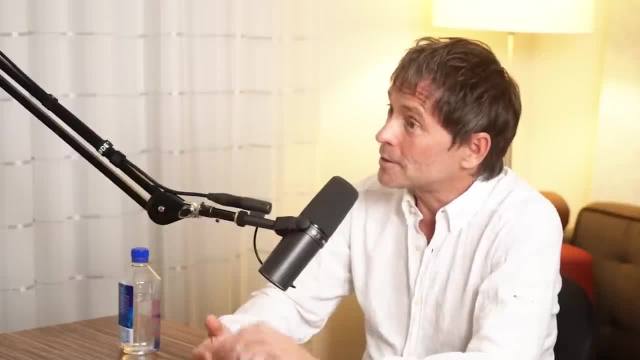 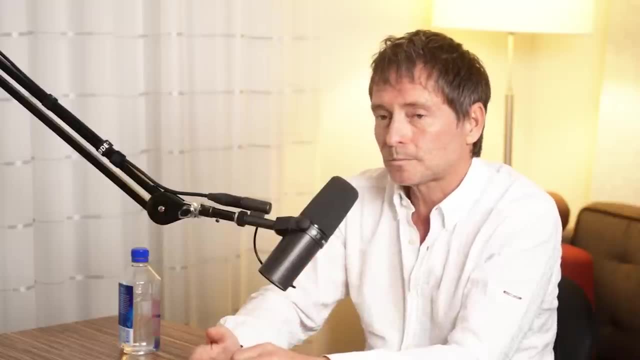 It's really incredible. So this was a revolution 1931, a revolution in logic, a revolution in mathematics, and we're still feeling the tremors of this discovery. So, at the end, it's a revolution, It's a revolution. 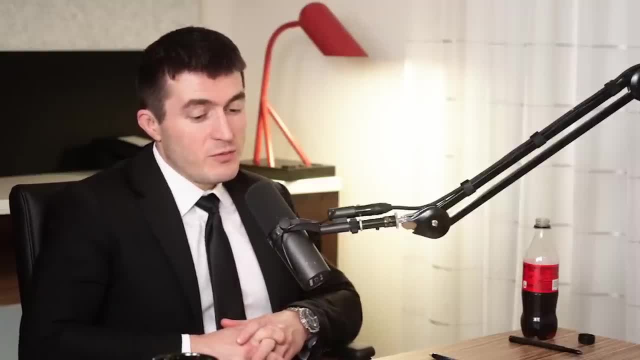 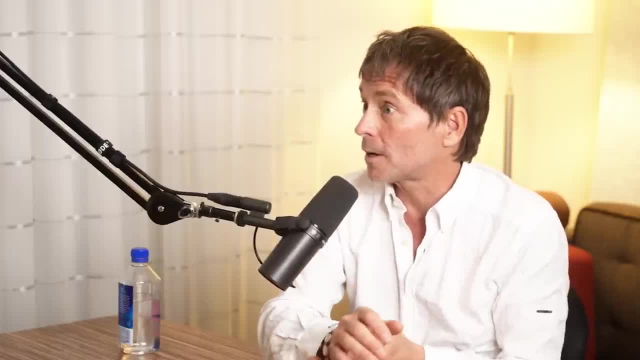 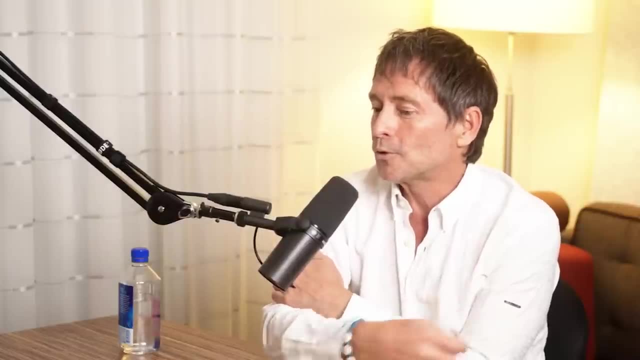 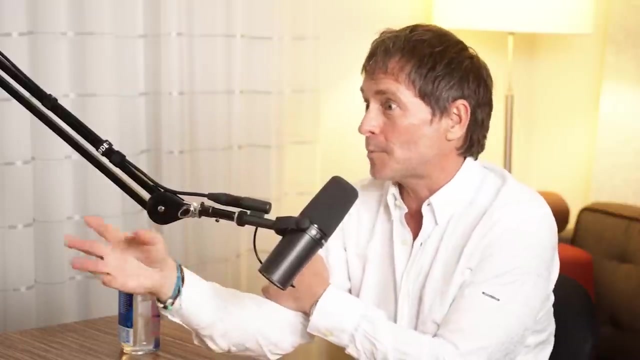 right. So he actually did something very similar. So he had this halting problem. He proved that halting problem cannot be solved algorithmically, that you cannot out of all computer programs. roughly speaking, you cannot have an algorithm of choosing out of all possible computer programs which ones are meaningful, which ones will not, which. 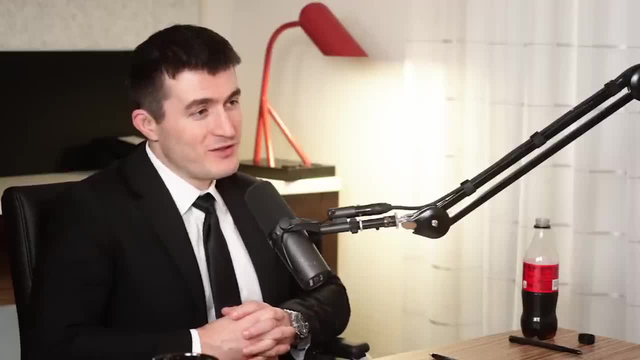 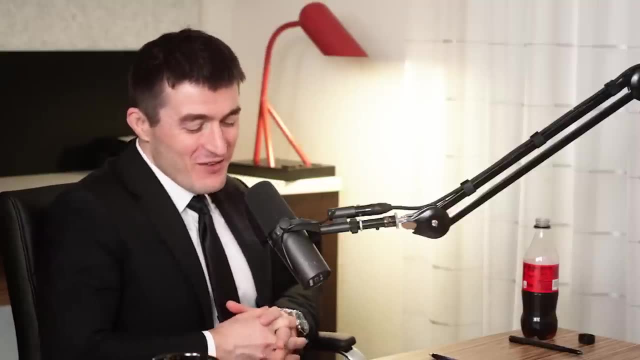 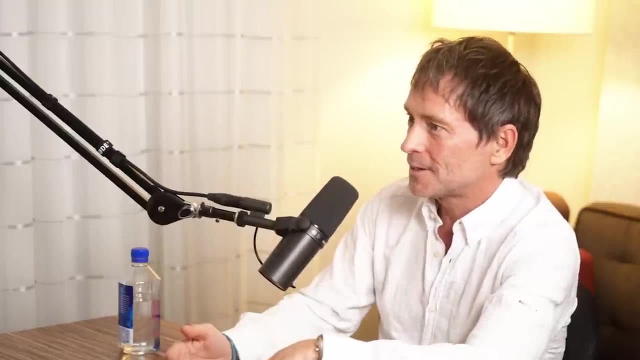 ones will halt Very depressing results all across the table. Or, on the contrary, life affirming depends on your point of view, Because everything is full of paradoxes. So that means so you're right. It's depressing if we are sold on a certain idea from the outset and then suddenly this: 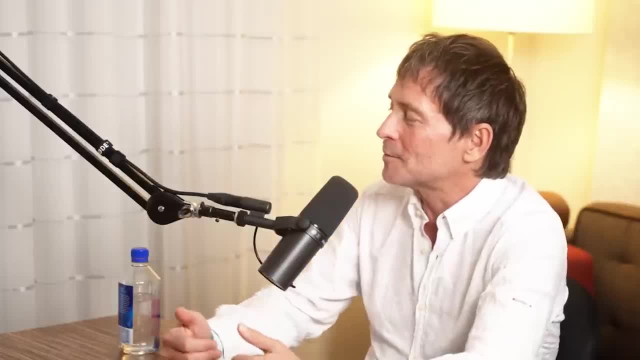 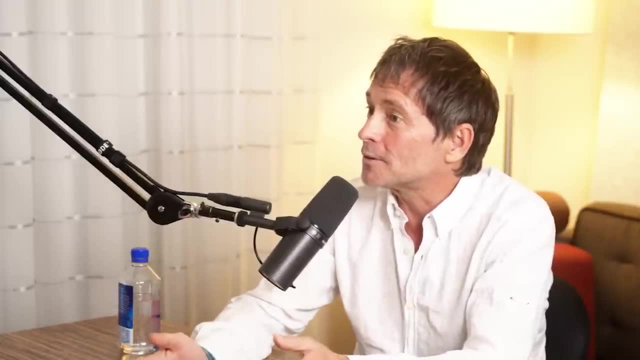 doesn't pan out, But okay, To which I retort. What if? What if he proved that actually everything can be proved? So then what? What is left to do if you're a mathematician? So that would be depressing to me. 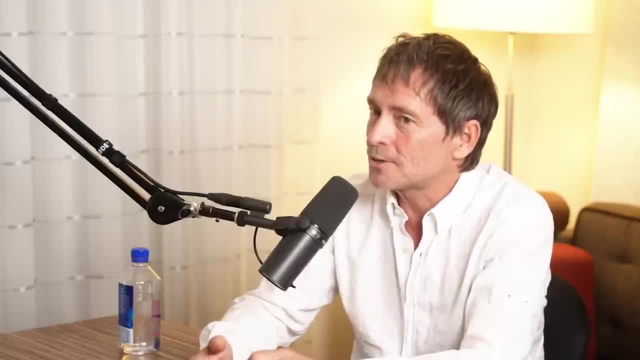 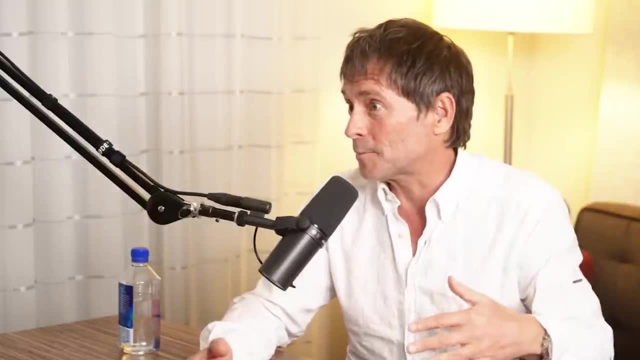 And here there is an opportunity to do something new, to discover something new which maybe a computer will not be able to Again, with a caveat: according to our current understanding, maybe some new technology, some new ideas will be brought into the subject. 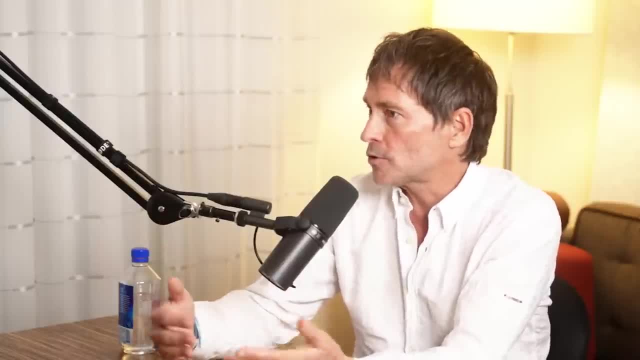 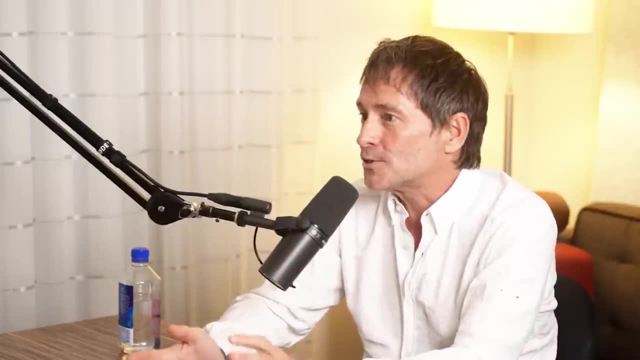 And the meaning of the word computation. like now we think of computations. Computation is a particular framework- Turing machines or church thesis and stuff like that. But what if in the future another genius like Alan Turing will come and propose something else? 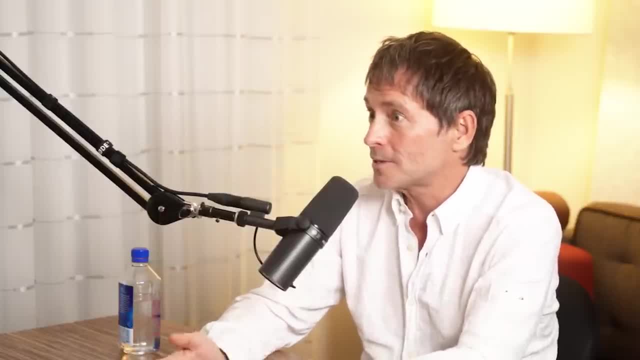 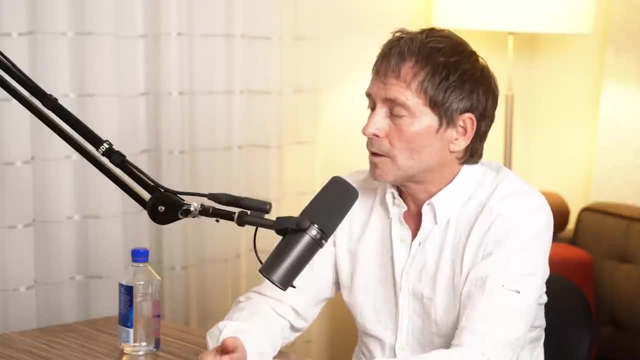 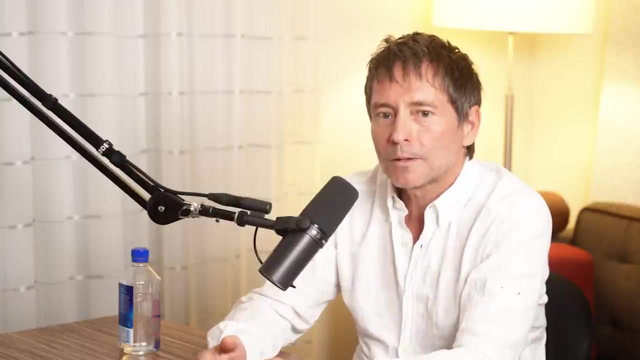 The theory will evolve the way we went from Newton's gravity to Einstein's gravity. Maybe in the framework of that concept some other things will become possible. So it's not. To me it's kind of like Not so much about deciding once and for all how it is or how it should be, but kind of 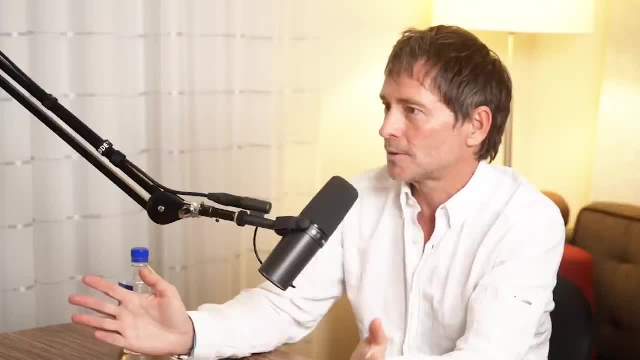 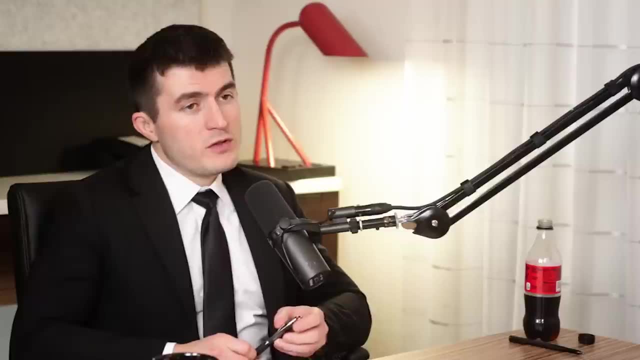 like accepting it as an open-ended process. I think that's much more valuable in some sense than deciding things one way or another. I wonder- I don't know, if you think or know much about cellular automata and the idea of emergence. I often return to Game of Life. 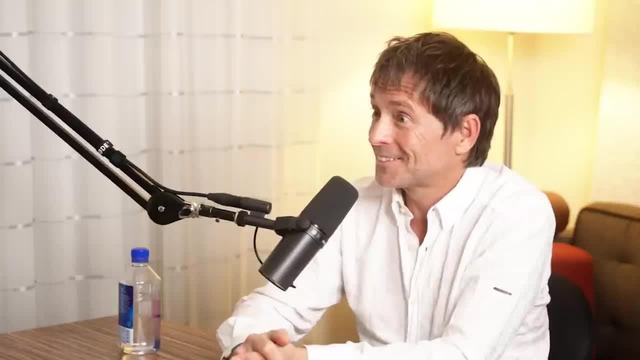 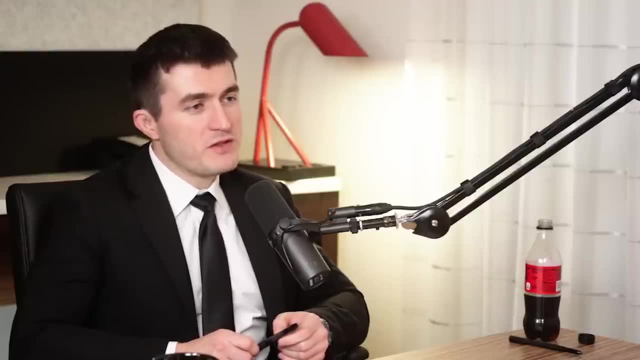 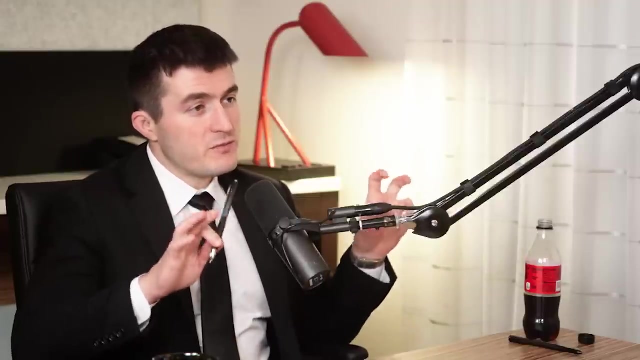 Yeah, And just look at the thing, Amazing right, And wonder The kind of things you can do with such a small, you know tools From simple rules. a distributed system can create complex behavior And it makes you wonder that maybe the thing we'll call computation is simple at the base. 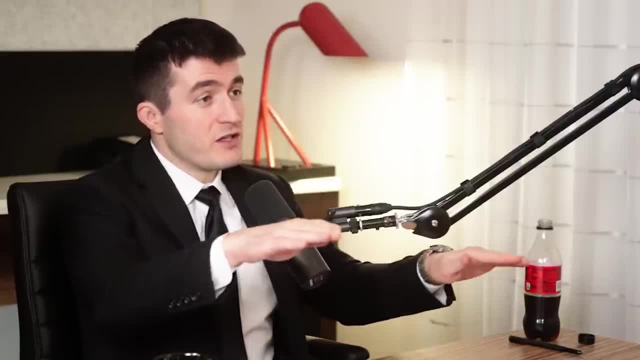 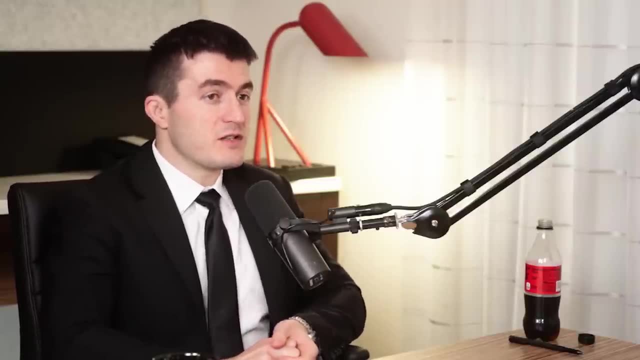 layer, but when you start looking at greater and greater layers of abstraction, you zoom out with blurry vision. Maybe after a few drinks you start to see some Something, Something that's much, much, much more complicated and interesting and beautiful than the original. 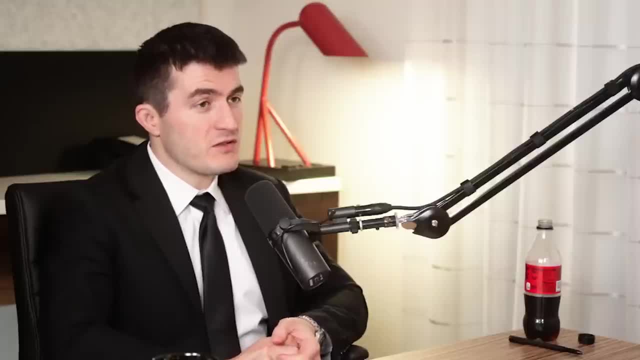 rules that our scientific intuition says cannot possibly produce complexity and beauty. I don't know. I don't know if anyone has a good answer, a good model of why stuff emerges, why complexity emerges from a lot of simple things. It's a why question, I suppose, not a 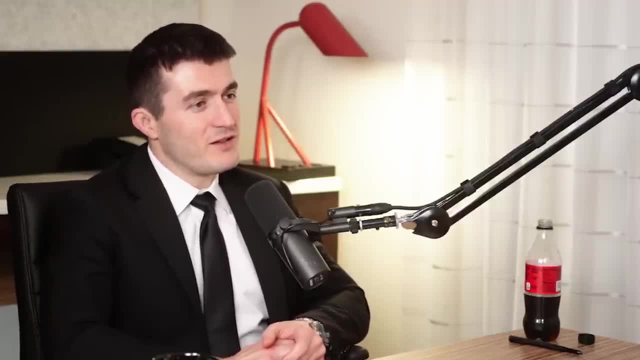 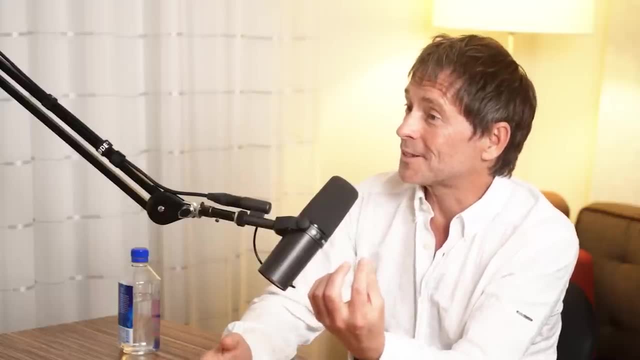 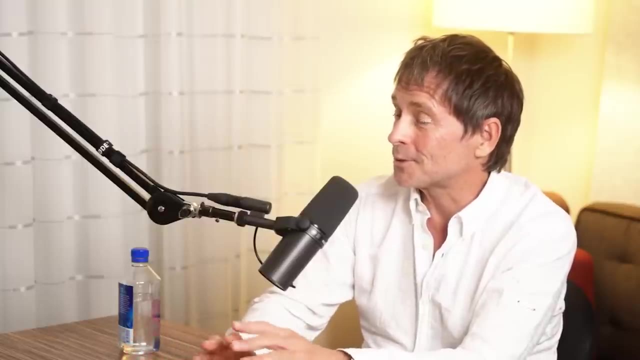 But every why question will eventually have a A rigorous answer. Not necessarily We could have an approximate answer which still eludes something Like quantum mechanics, 99%- Maybe We'll be able to describe it with 99% certainty or 99% accuracy. 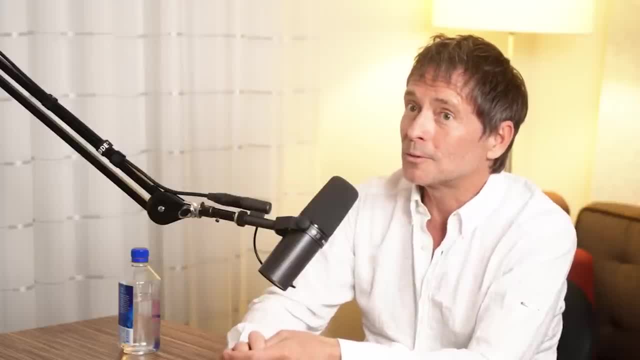 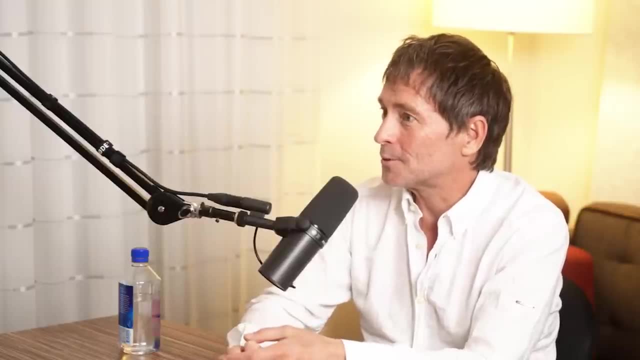 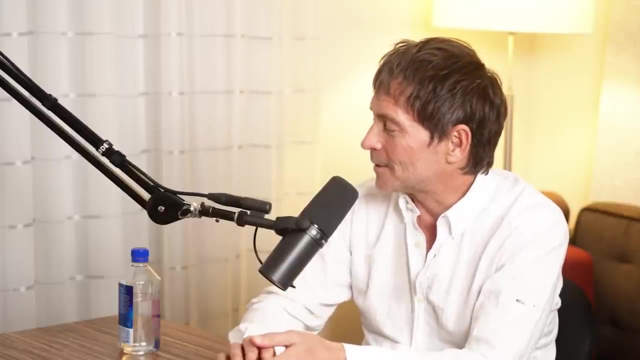 Yeah, And then maybe, you know, in a hundred years or, you know, next year, somebody will come up with a different point of view which suddenly will change our perspective. Yeah, You know. to this point I want to say also: you know one thing that I find fascinating. 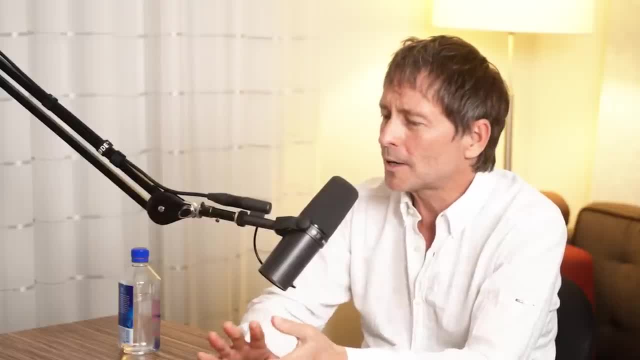 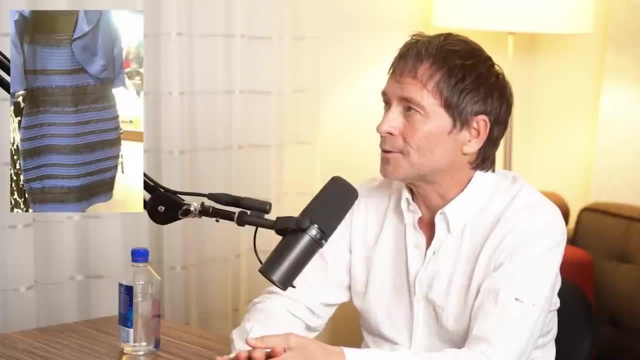 speaking of paradoxes and so on, Do you remember how everybody was freaking out about this blue dress And the blue? Was it blue or was it black? Yeah, It was, I think yellow and white, or black and blue, Mm-hmm. 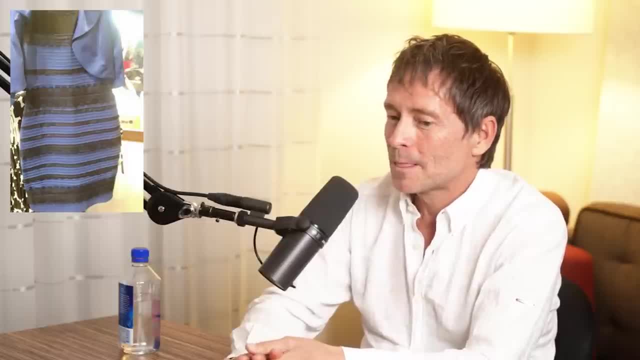 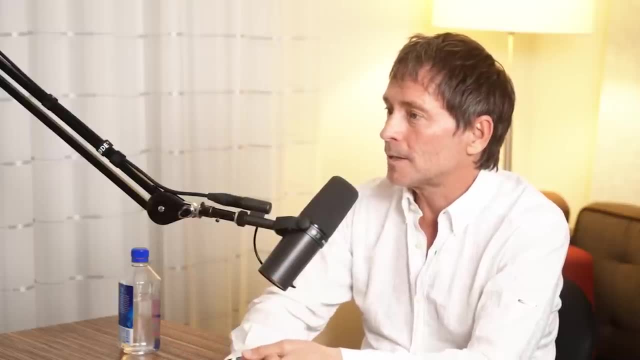 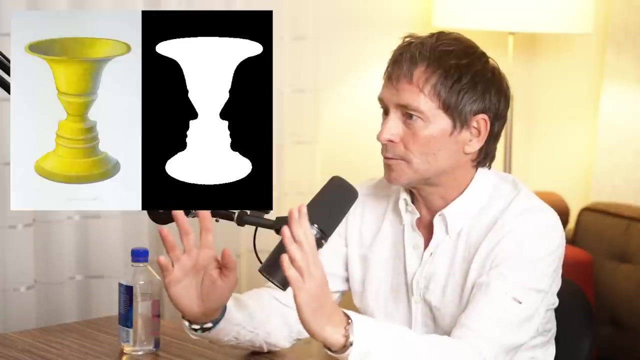 It almost broke Twitter. Yeah, You know, I remember that. Yeah, That night. So there are many examples like that where you can perceive things differently and there is no way of saying which is correct and which is not. For instance, you got this, the vase, the Rubens vase. you know where you have from. 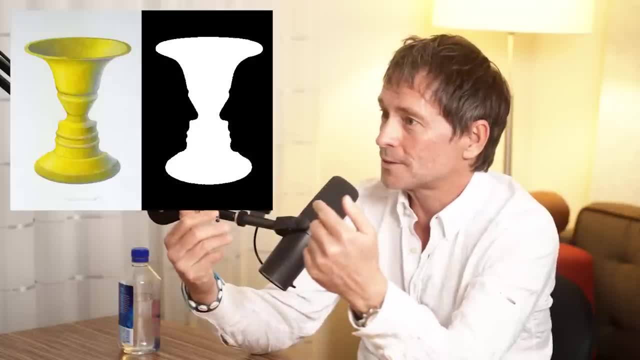 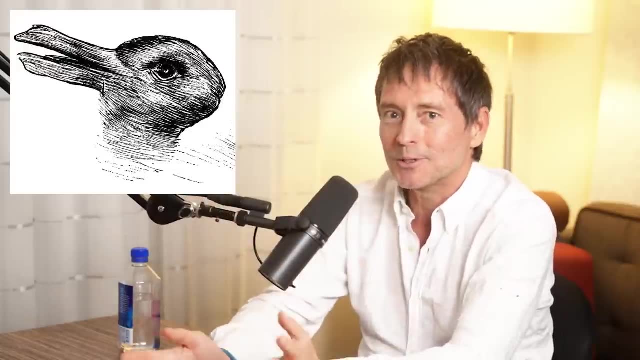 one perspective it's a vase. From another perspective it's two faces. Then there is this duck-rabbit picture where you can Google it. If somebody doesn't know, they can Google it and find it. It's very easy. 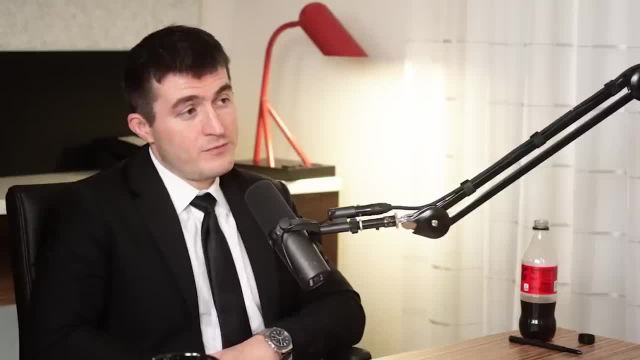 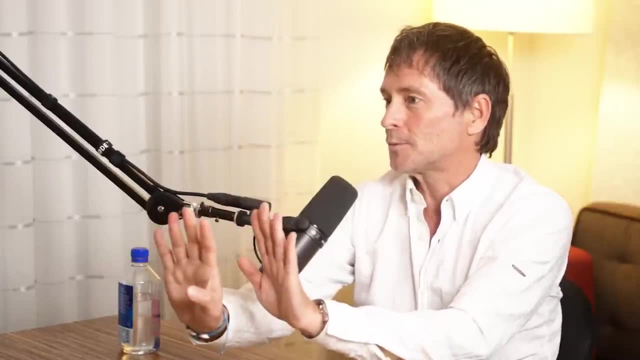 Actually, Ludwig Wittgenstein devoted several pages duck-rabbit in his book, And so on. There are many others. There are like squares where you can- A square you can see from different perspectives This way, that way, and so on. 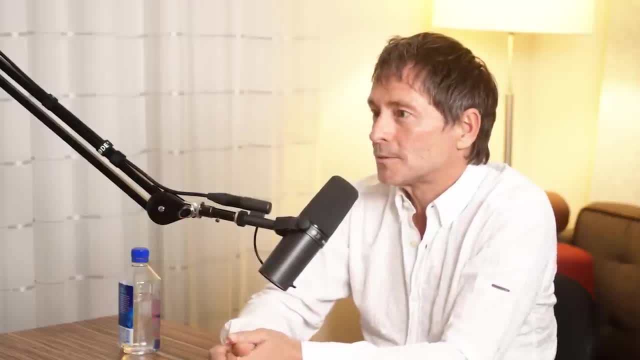 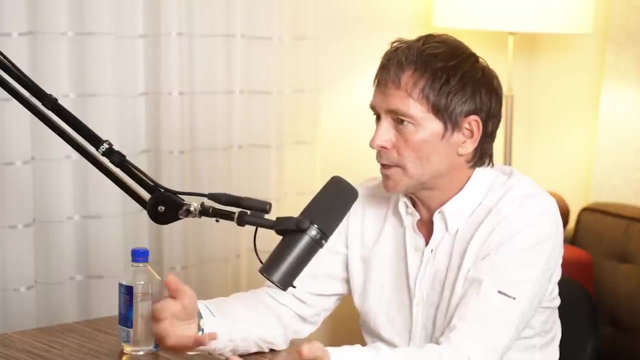 So when we talk about neural networks, we're talking about training, data and stuff, so that you have some pictures, for example, that you feed to your program and you try to find the most optimal neural network which would be able to decide which one is it the. 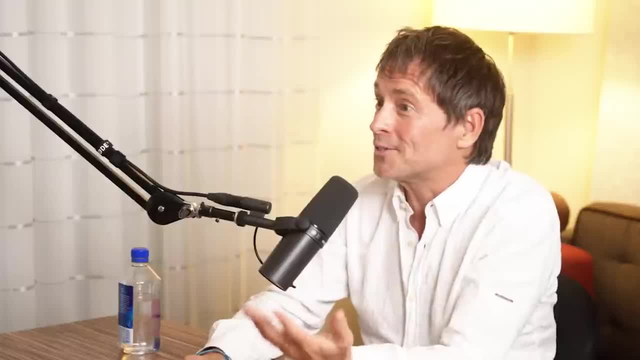 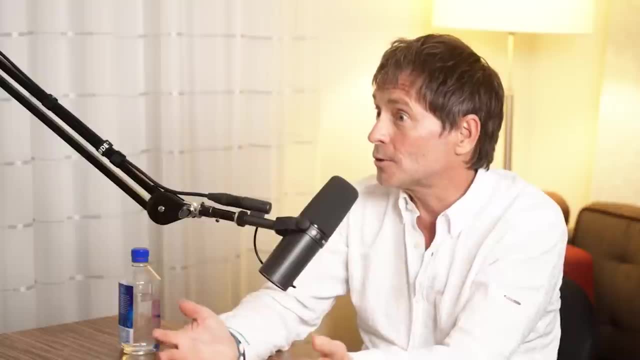 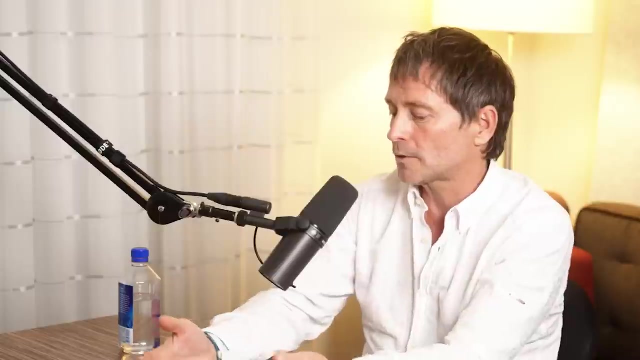 dog or a cat or whatever, But sometimes it doesn't have a definite answer. So what do you do then? So actually it's a question I actually don't know. Has modern AI even come to appreciate this question, That actually sometimes you can have a picture on which you cannot say what it is in it? 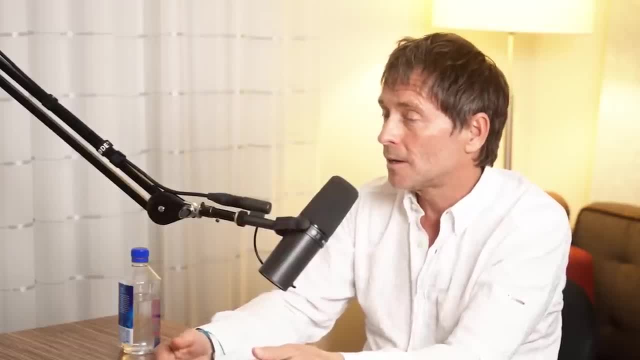 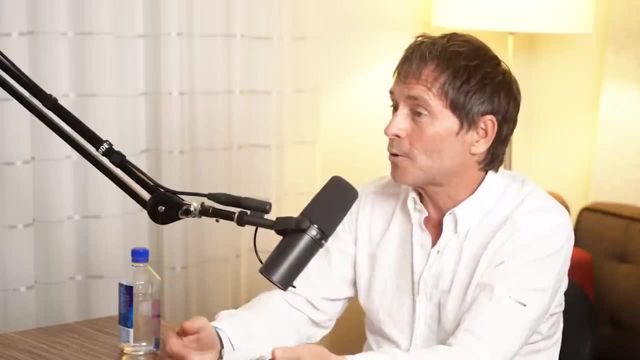 From one perspective it's a rabbit, From another perspective it's a duck. How are you supposed to train If you have a neural network which is supposed to distinguish between ducks and rabbits? how is it going to process this? you see, 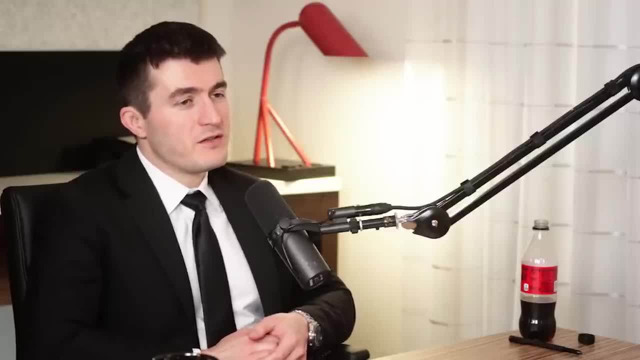 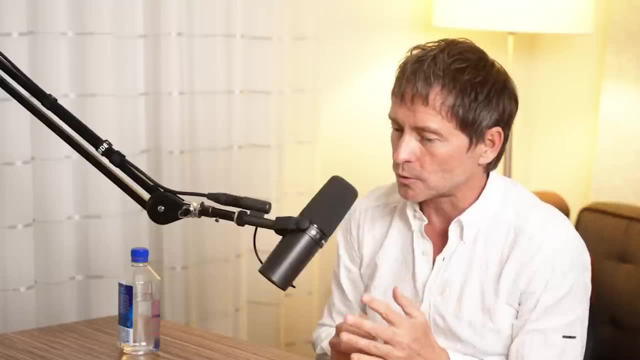 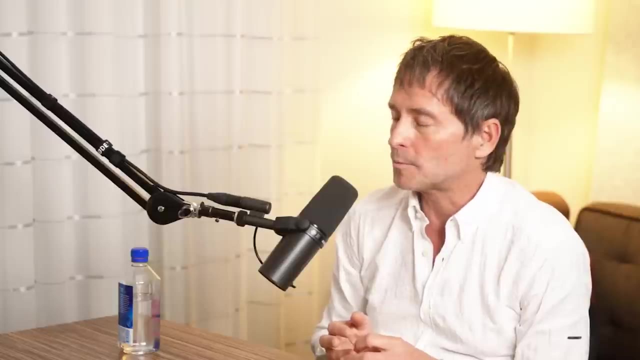 Well, So the trivial trick it does is to say there's this X probability that it's a duck and this probability that it's a rabbit. That's a good approach, But also I would say there is no given percentages, For instance. actually, at some point I was really curious about it and I looked 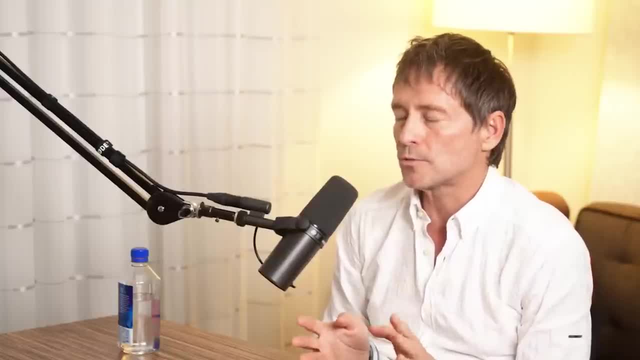 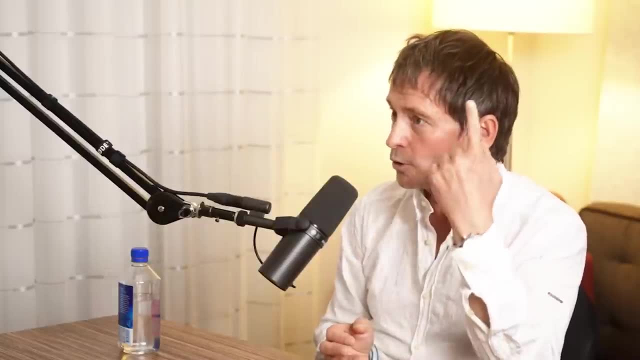 And for each picture of this nature- and there are a bunch of them you can easily find online- my mind immediately interprets it in a particular way: Mm-hmm. But because I know that other people could see it differently, I would then strain. 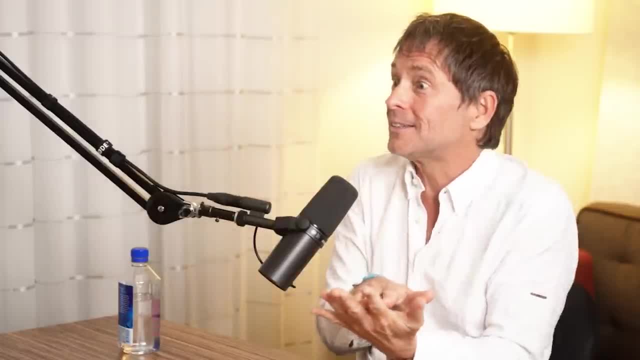 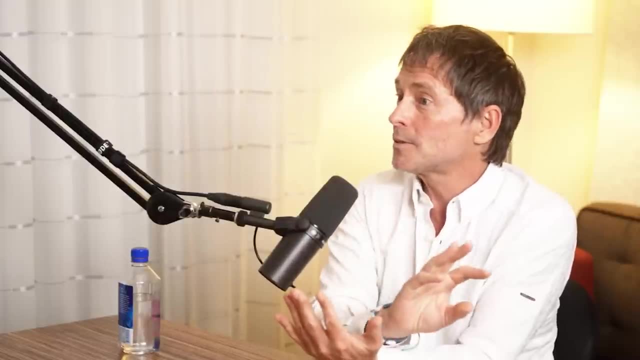 my mind and strain my eyes and stare at it and try to see it in a different way, And sometimes I could see it right away and then I could go back and forth between the two And sometimes it took me a while for some pictures. 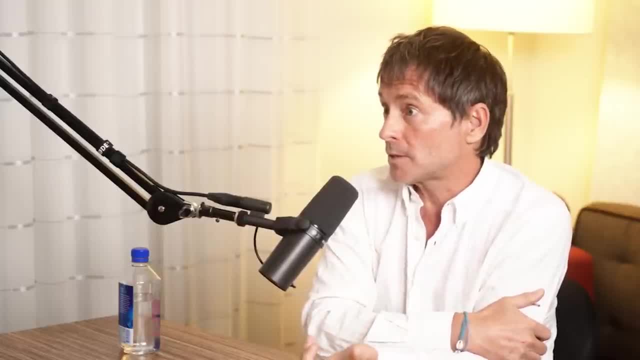 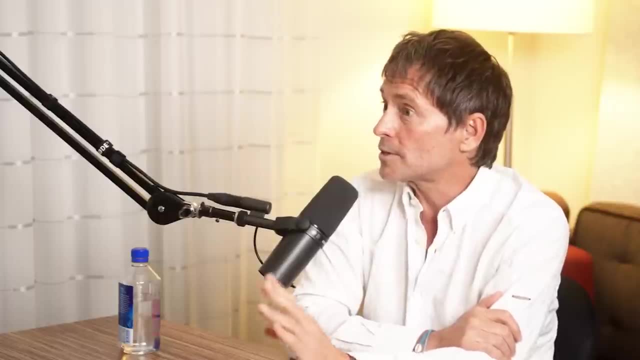 So, in that sense, even if these probabilities exist, they are subjective. Some people immediately see it this way, some people immediately see it that way, And I think that nobody knows- Not psychologists, Not neuroscientists, Not philosophers- What to make of it. 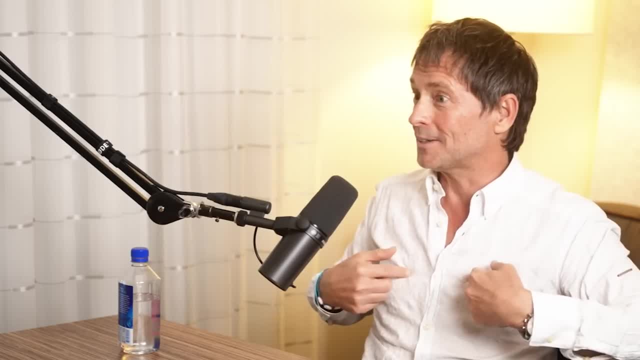 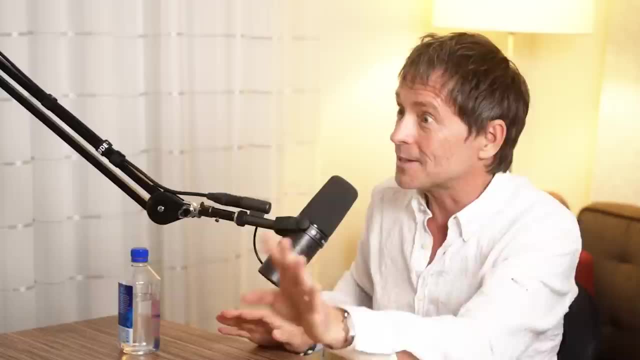 The best answer, of course, as a scientific mind, even though I say no, don't look for interpretation, leave some place for mysticism or mystery. right, I say that, But of course I want a theory, I want an explanation. 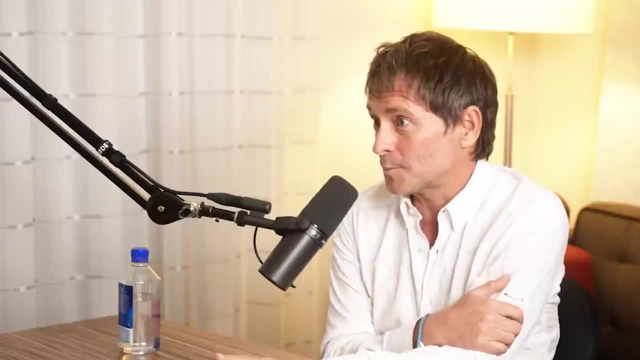 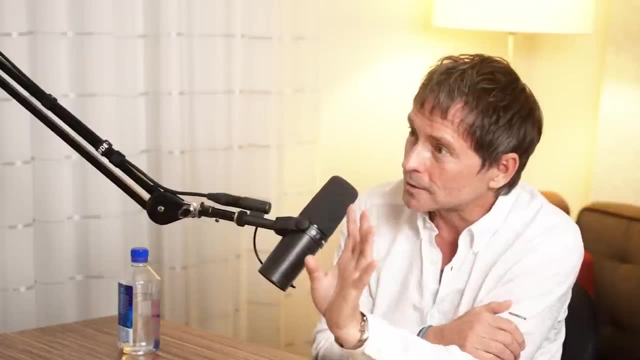 So the best explanation I find is from Niels Bohr's complementarity principle. So it is like particle and wave, that there are different ways to look at it, and when you look at it in a particular way And the other side will be obscured. 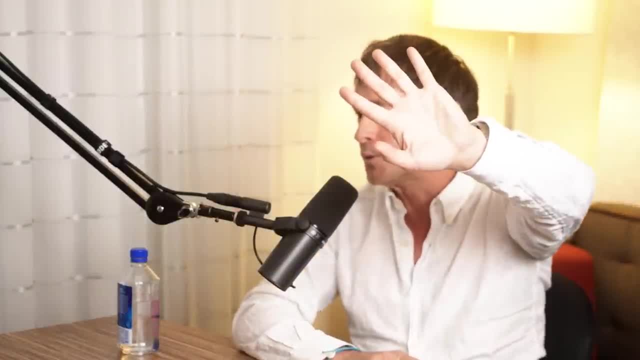 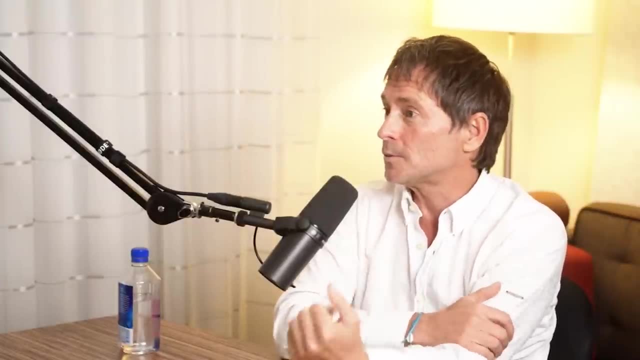 Think about it like the other side of the moon, So we are observing the moon from one side and then we don't see the other side. There is a complementary perspective where we see the other side but not the side we normally see. 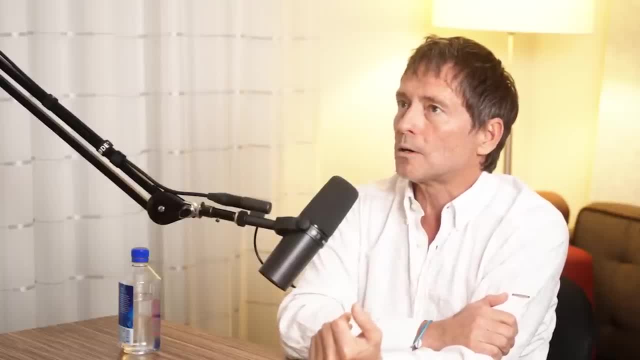 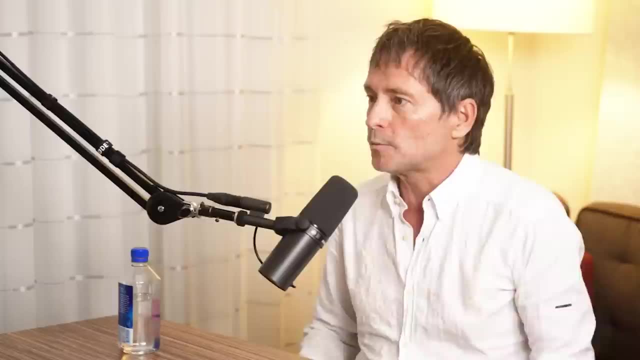 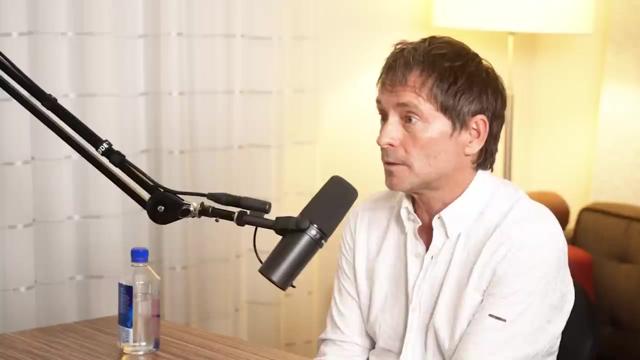 But the moon is the same, It's still there. It's our limitations of being able to grasp the whole. That's complementarity, And we know that from quantum mechanics, that our physical reality is like that, rather than being certain, Rather than being one way or another. 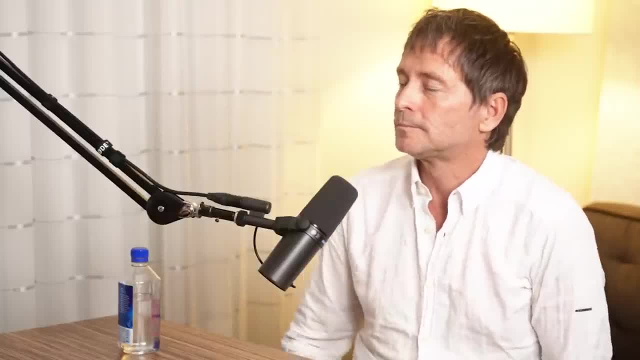 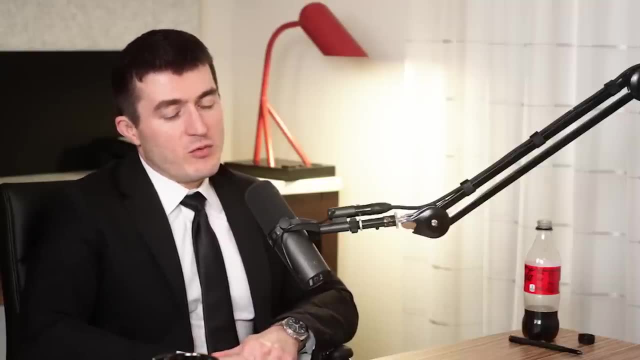 We should, just as a small aside in terms of neural networks, mention that at the end of the day, there's humans. it's built on top of humans, Or with ChatGPT, that is, using reinforcement learning by human feedback, we're actually 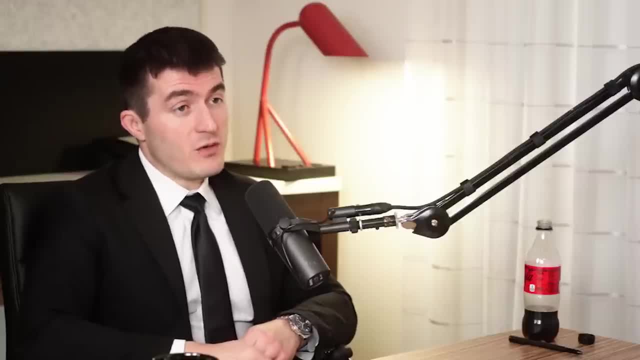 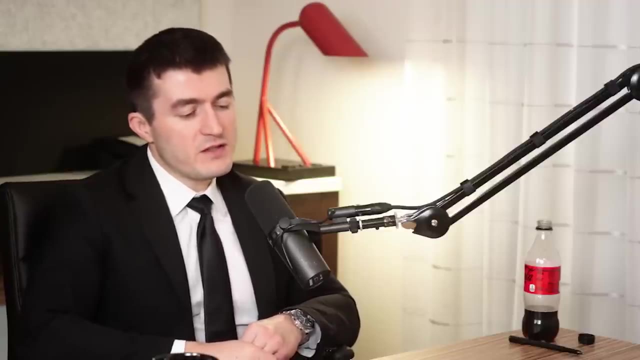 using a set of humans to teach the networks, And that's the thing that people don't often talk about, Because- Or Let's think about that- Those humans all have a life story, Each human that annotated data, that fed data to the network or did the RLHF they have. 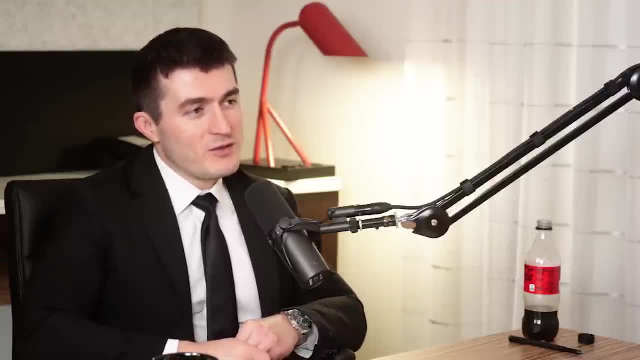 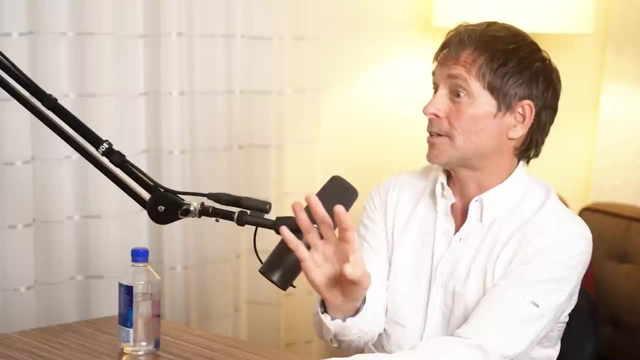 a life story. They grew up. They have biases. They have biases. There's some things that they like, there's some things they don't like, which can kind of appear under their radar screen. They may not be aware that they are exercising those biases. 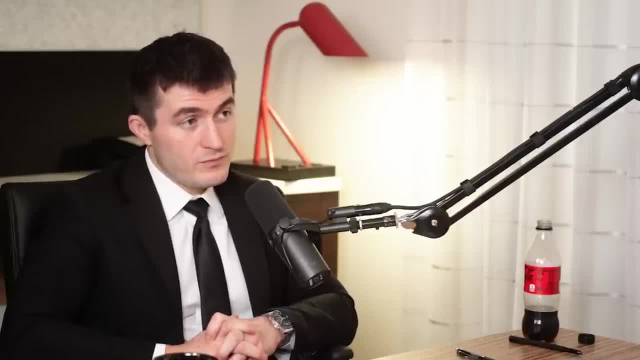 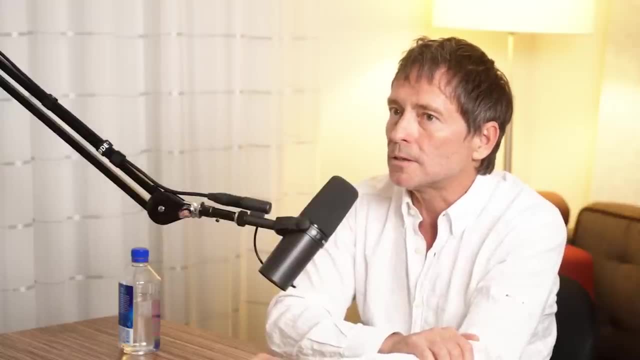 That's the point. What you brought up is a very important issue here. Not so much issue, but it's not a bug, It's a feature. in my opinion, That, implicit in the discussion of the question is thinking, computational and so on, is the. 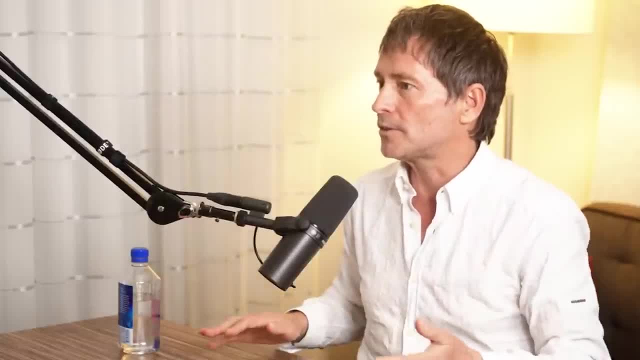 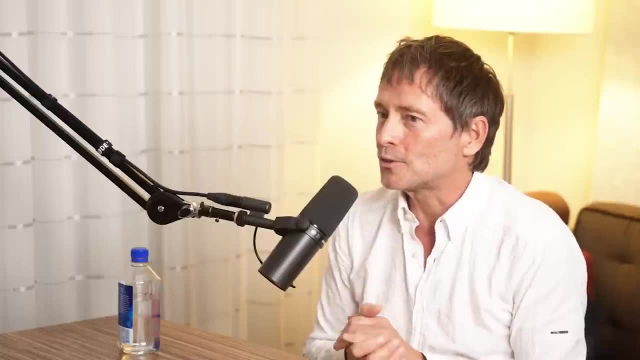 idea that our conscious awareness covers everything within our psyche, And we just know that that's not the case. All of us have observed other people who have had sort of destructive tendencies, So obviously they did things destructive for themselves. Yeah, Yeah. 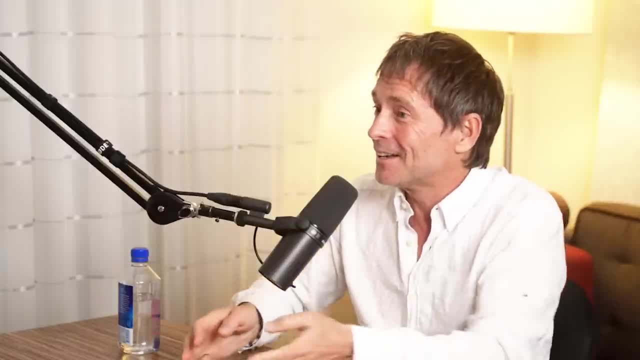 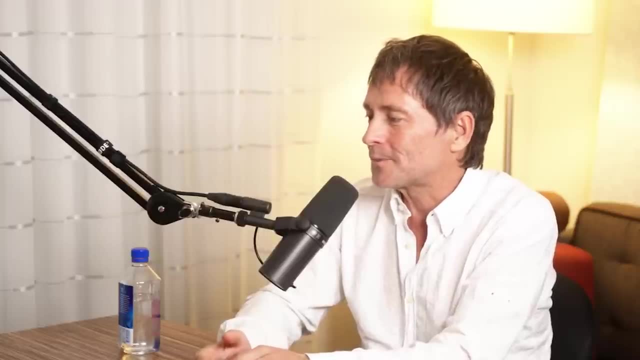 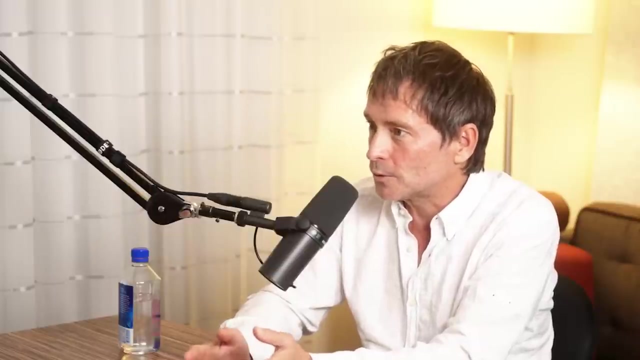 And many of us have observed ourselves too doing that as part of human nature. right, And there is great research in analytic psychology in the past hundred years strongly suggesting, if not proving, the existence of what Carl Jung called the personal unconscious, and also 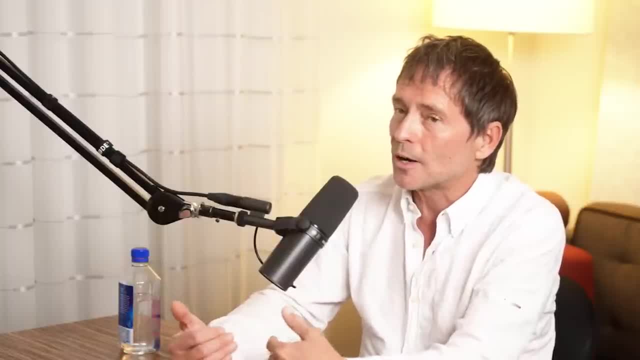 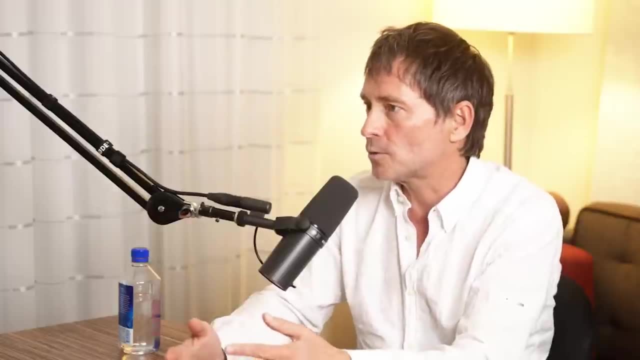 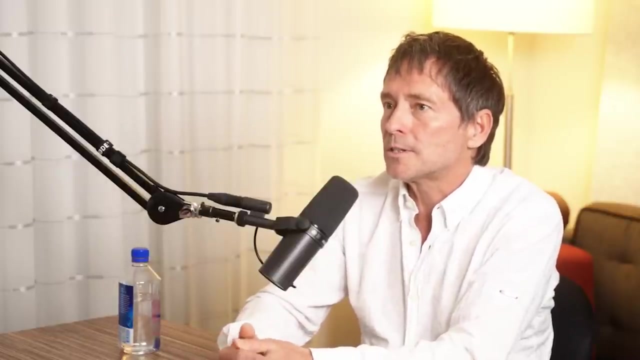 collective, unconscious, This kind of circle of ideas which are under the radar screen, which lead us to some strong emotions. They require us to act in certain ways, even if we cannot really understand. So if we accept that, then the proposition that somehow everything can still be covered. 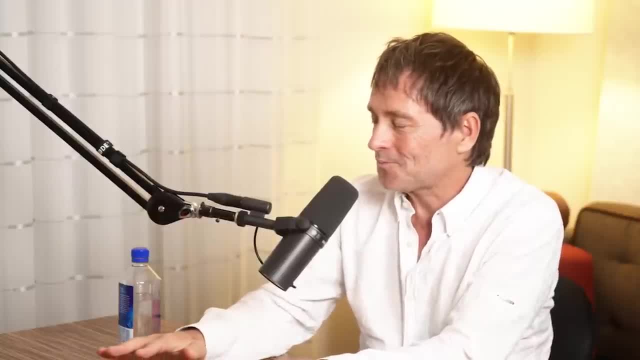 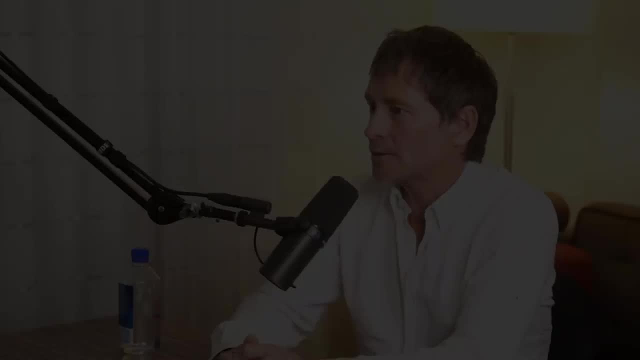 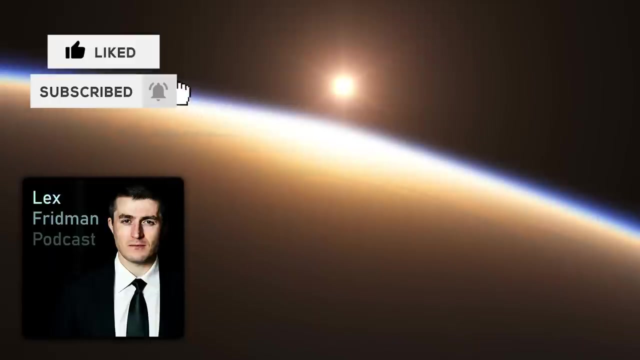 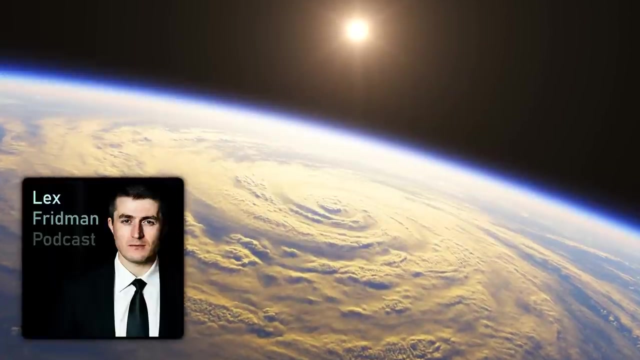 by our actions, which are totally neutral and totally righteous and totally conscious, that it becomes really tenuous. So that's what I'm asking…. Yeah, …is an old saying, Yeah, …in the life of a soul, Yeah, 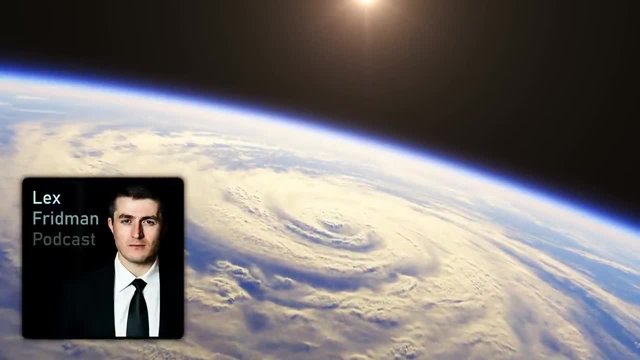 But you may have heard of it, but not immediately. Maybe not until you get to say nine years or so before you discover that you are actually human, You got to get out. Yeah, Yeah, You got to get out. Yeah, You got to get out and reveal that you are as you see fit, right, That kind of thing is. I don't know, And you're going to feel it because you get to feel it. That's the secret of you know, being an inner soul. It's different, It's like, you know, like this is like that, It's not going to be out now, My god Yeah. 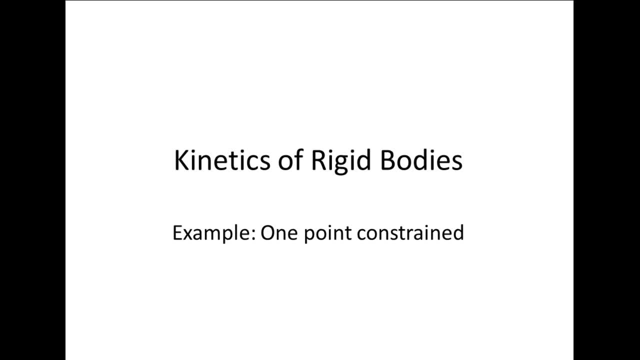 In this example we will examine a rigid body problem in which one point on the body is constrained to move in a certain direction. A slender rod of length L and mass m has a roller attached at point A. The rod is released from rest in a vertical position with the roller on a surface that is inclined at an angle- theta.